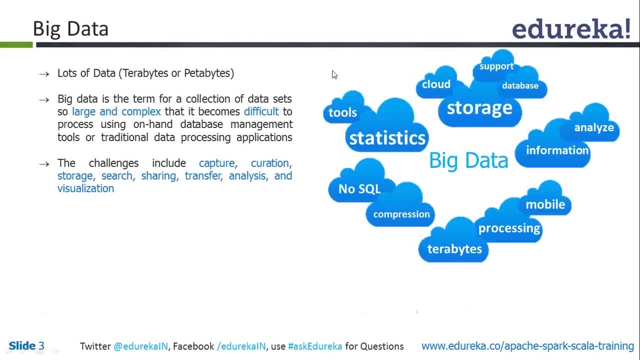 So I'll just give it a name: back And after that去, quick view and all that. if the database file size of whatever database you are handling with is in the order of several GBs, then you are actually talking about a big data instance, a quite a big data instance. altogether right, but right now. 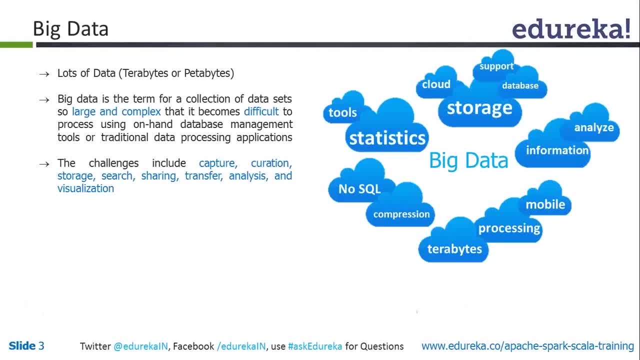 that is scale. so three, four years, you know, earlier the scale was at several GBs. right now as kind of an industry standard, and I'm not talking at the level of Facebook and Google who have moved to the petabyte scale, but at the industry standards. high side of GBs means, you know, 500 GB, 600 GB, kind of. 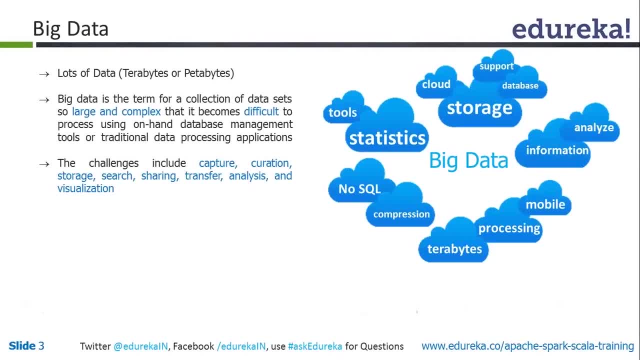 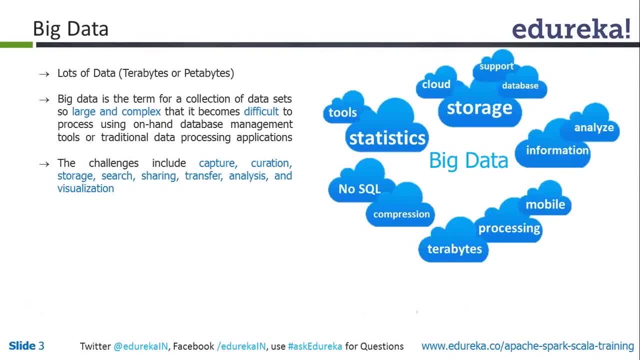 all together different. there are some other aspects, which are you know which, which come along with it. you must have heard, or heard about, you know, that famous 3d thing altogether: volume, velocity and then variety. I will come to that part because that's more of a theoretical nothing it's all about. 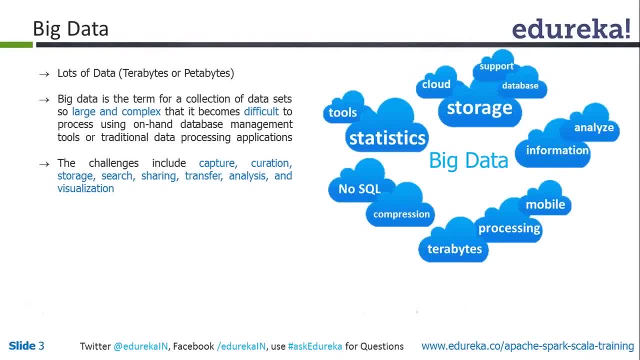 reaching that point and there is, when you have so much of data, then it becomes very difficult or sometimes almost impossible to handle it with the traditional applications all together, or that traditional monolithic, you know, service or applications which tend towards the vertical scalability. when you talk about vertical scalability or talking about increasing the strength of 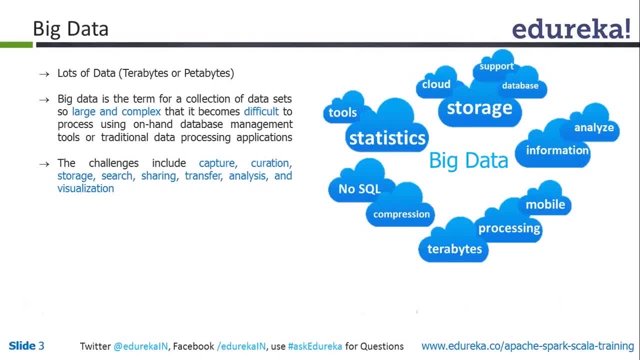 can have more processing power altogether, invest more money, keep on increasing this trend, but again, there is a limit to it, so sorry. typically all of the distributed uh processing systems, they uh work on the horizontal scaling side, wherein they say, okay, we are not really going to invest too much. 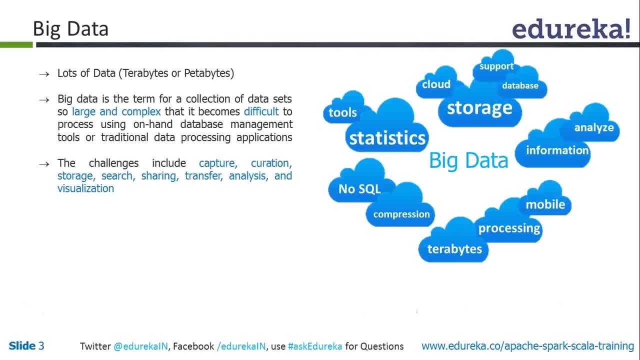 on each and every machine. instead of that, can we have a cluster of you know, some relatively cheap machines- uh, they are typically called the term for that is commodity hardware. and can we do the distributed processing to achieve the same results in much lesser investment altogether, of course it. 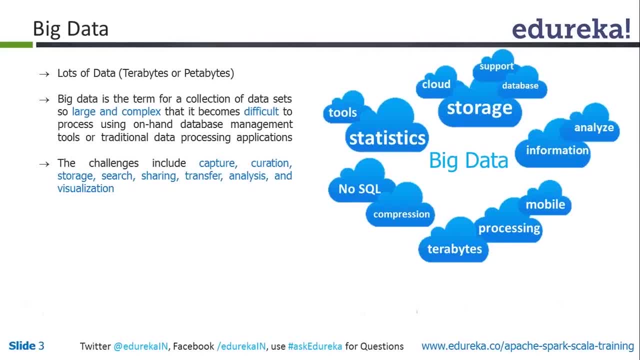 leads towards, you know, its own challenges. so those, apart from those 3d challenges which you must have heard about: volume, yes, velocity, at the rate it which at which you know you are capturing the data, or probably processing the data, and variety. when you talk about variety, it is about you know, 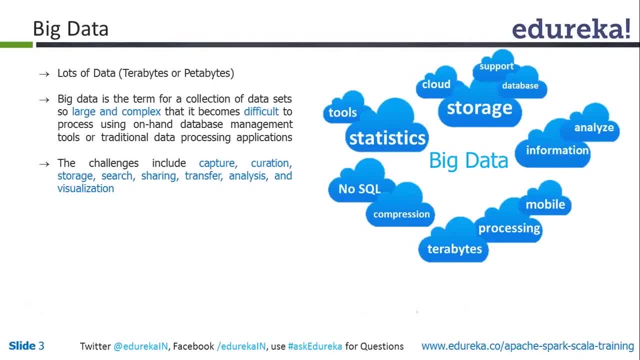 uh, you are dealing with structured data, unstructured data, semi-structured data. apart from these three v's, when you go to the distributed world, distributed processing world, which you you typically use for the big data you are, you encounter different kind of challenges altogether. you talk about distributed processing, then how exactly you are going to maintain the 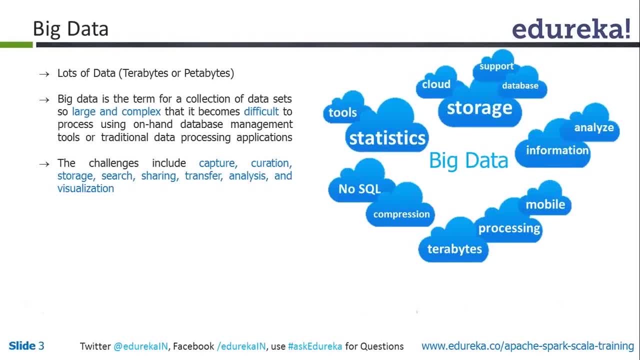 states how exactly you are going to, you know, deal the failures, or probably partial failures, then fault tolerance and all all those things come, you know, bundled along with it. so these are some of the factors, again at the very, very high level. these are some of the factors which make your big data world completely different from a, from the 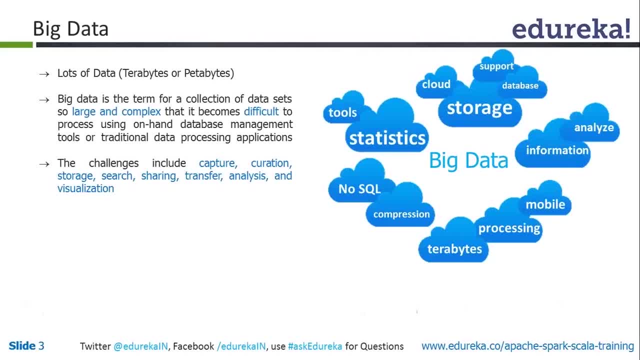 perspective of your traditional world as such. okay, the challenges. of course you are dealing with such a huge data. repeat the capturing side of it, be the data messaging side, be the sharing of information transfer, analysis, even the visualization right. so all of these things face those typical challenges. your typical way of working doesn't really hold anymore. yeah, right, 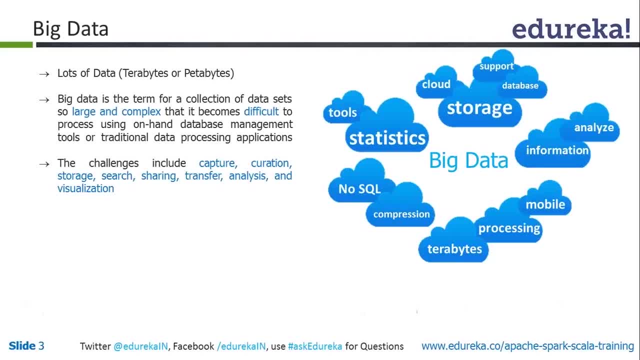 because you cannot really, uh, perform a select star from a specific table, whereas that table is having, let's say, around billion records. right, so you are. you are not going to get fast responses. that's the simplest example, but, yes, there are various others, so i would not spend much time on this side. i hope you would have. 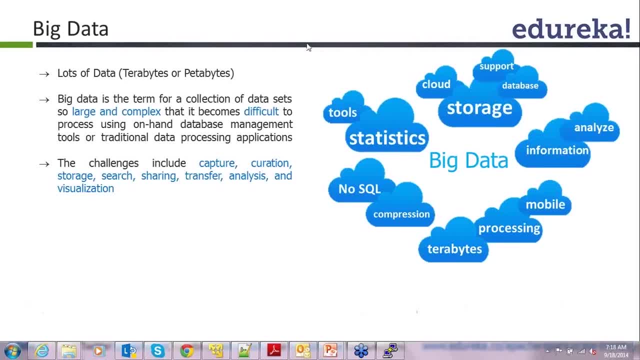 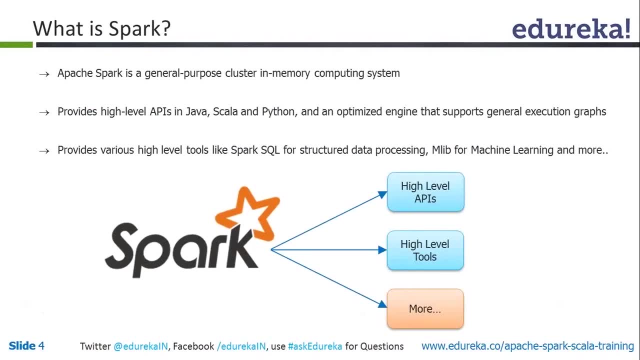 got some idea about kind of you know challenges which are involved here right now. let me come directly to spark before this. uh, just for the people who don't know uh about, you know big data world. i would highly recommend, if you could, you know, spend some time on, uh, you know google or wherever you know study material, just see. 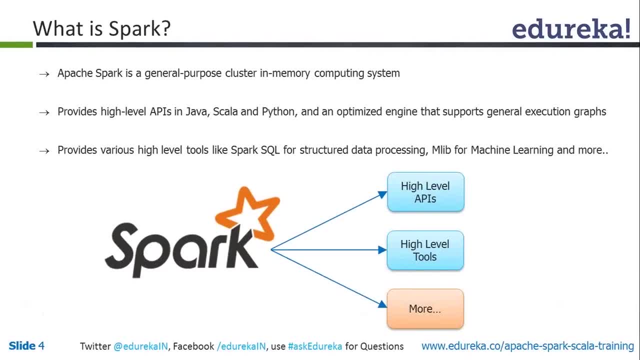 what exactly do you mean by the batch with data processing? see, batch processing is one and batch big data processing is other. there is a difference. and then, uh, something called lambda architecture. okay, that would give you good idea about why exactly you should even go for something called spark or something like that. so i would recommend you to go for something called spark. 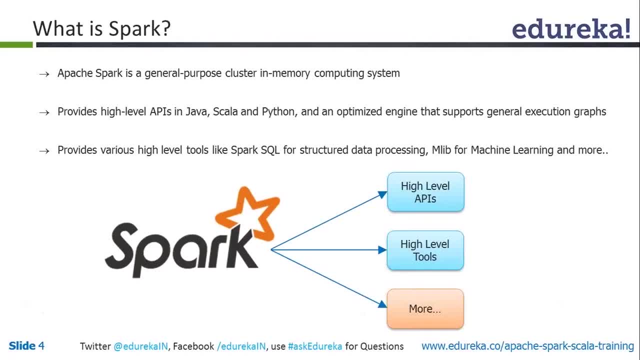 supply data processing from spark, Sandy or sams as comic Его- myself, or you may also want to- à, then it's permissible to go for some reason. what so? what's the thing that i like to think which need to be improved? two is teamwork, which maybe you're used to as a pharma company, is had this kind of thing where it would lead to pooling or storm, so aẤ are probably storm, so uh, coming to. so this is something which i would leave for those people, uh, who are not aware of this. now, coming to sport, spark is typically used for near real time processing or for a very fast patches or the time good party. okay, now, before coming to what, where it. 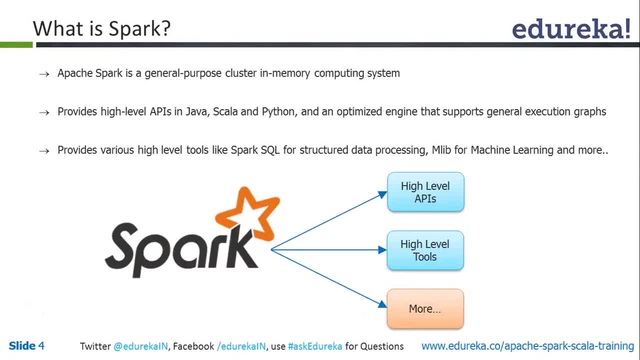 is it so as the first line says? now, I'm not. I'm not a fan of reading out the slides, but sure since it's kind of a definition itself, right? so Apache Spark is a general purpose cluster in memory computing system. good, what does it mean? what does it mean? so let me just break it down. Apache Spark is a general purpose computing. 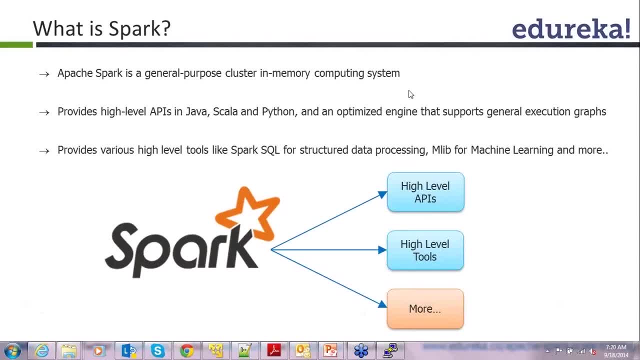 system, so must be sounding something like Hadoop right. general purpose cluster computing system means almost like Hadoop right, so it's a general purpose cluster computing system. you're talking about distributed processing and the moment you talk about cluster, most of the time it's more or less it is going to be commodity hardware and the only difference is it's in memory. 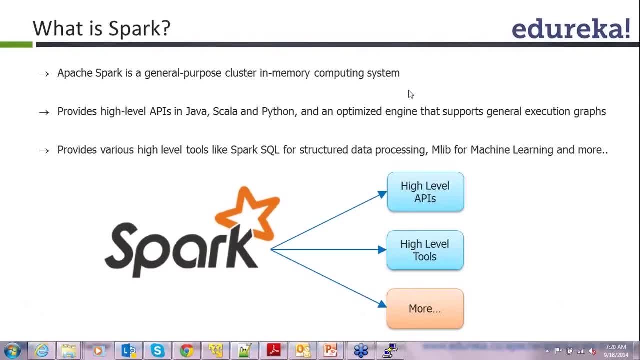 computing system. now, when you talk about in memory computing system, you typically are going to perform your calculations in the distributed fashion, but your operations are going to happen in memory, not really strict, strictly in memory. there are various options which are available. I'm sure those people who are from big data world must be thinking: what if you know my data, which? 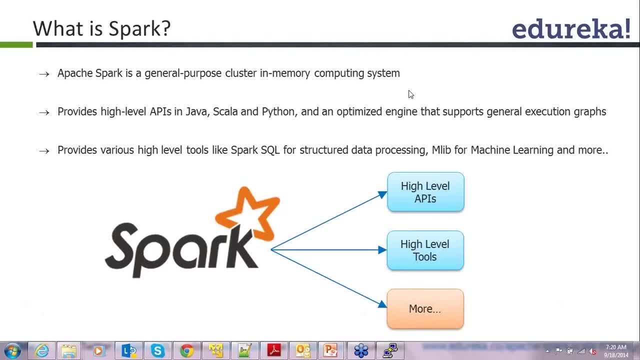 is there in Asperger's with? no, doesn't really fit into memory. I'm sure some of you would have thought about it, right, but for now just assume that, yes, it is going to fit, though there are, of course, in practical it is not, and then there are options also available for it. okay, so we can. 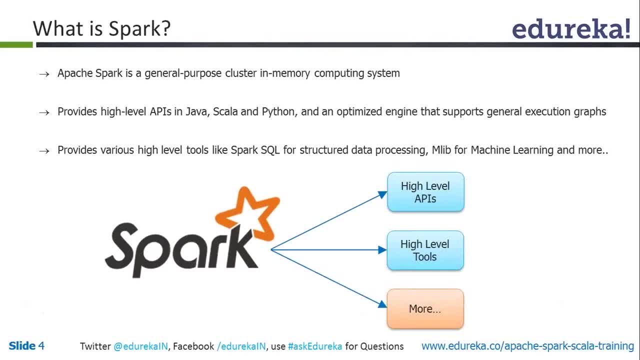 come to those parts when we'll be talking about when you know we'll be discussing spark and details in the classes, but for now it is the general purpose. cluster in memory computing systems. your most of the calculations happen in memory, altogether okay, and then this is one since. 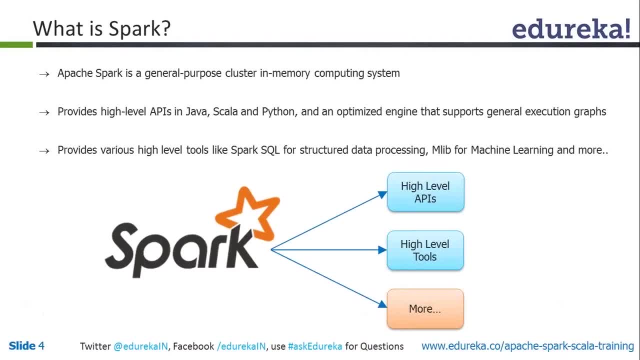 the calculations are going to happen in memory. they are going to be much faster because you are not reading the data, you are not doing the on-demand paging altogether. you are going to perform the calculations in memory. so they are going to be much faster than typically they are in hadoop. the other thing is you kind of 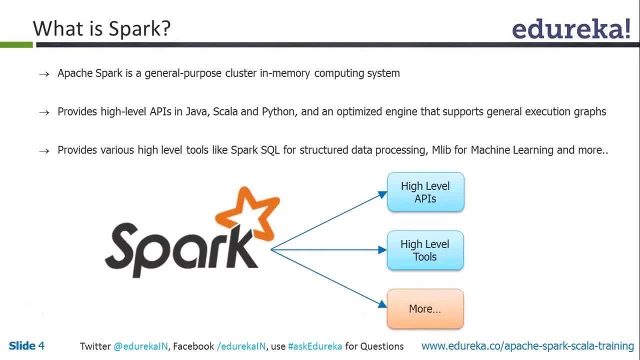 know all these things. you know I can't do that which. I've done, all these things together, and I don't know if this is a good policy, that I should be doing, or not I should be doing. I should be doing all these things together and then I can't do it. 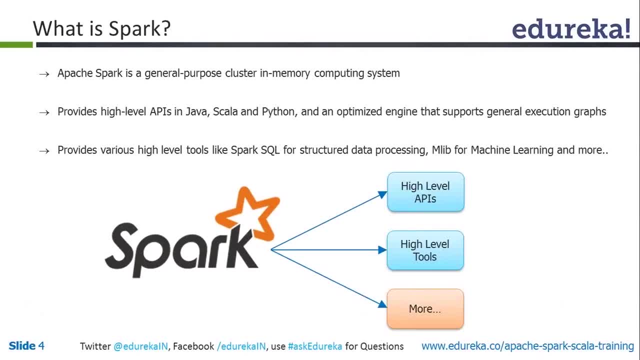 right. okay, in C++ or javascript, for that matter, not as of now, probably not as of now. probably there would be some support in future, but not right now. Now I will come to why exactly. on Scala and all. so it is quite an optimized engine, which. 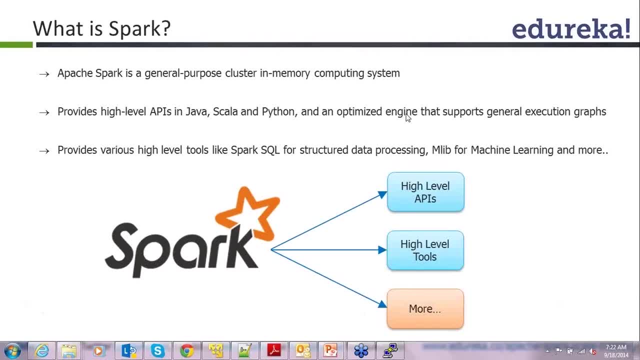 supports the general execution graph. again, its kind of a very abstract statement. its all about guys. that spark follows something called lazy evaluation all together and lazy execution its all about. if some of you have worked in peg, you must be knowing that it typically goes for the lazy processing until and unless you force an action, whatever calculation. 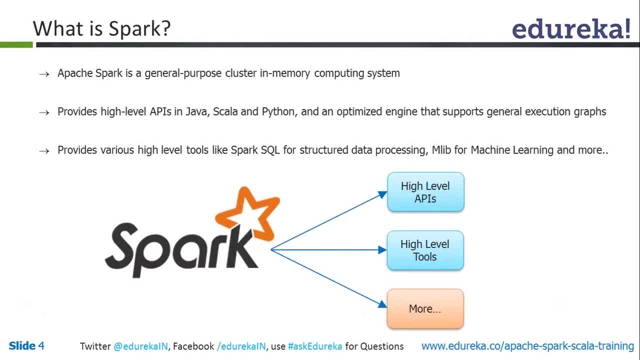 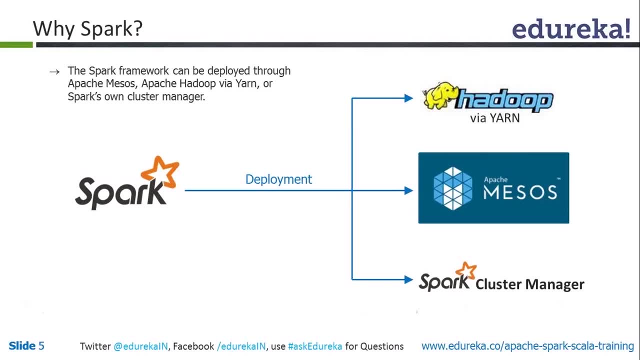 you have done. that is done logically. that is not actually invoked on the data, so that leads to a big, big performance optimization. all together, Ok, Now, these are the two points, but the third point is even more important, which differentiates the spark from others. so it is about spark provides you the high level tools like spark. 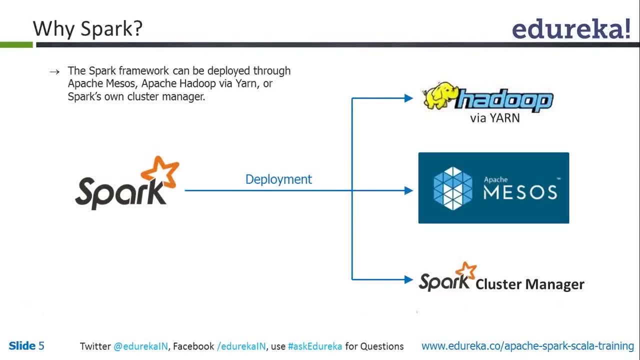 sql for structured data processing, mllib. there is a spelling mistake here. it is written as mlib, it is not. it is mlib: machine learning library for machine learning and more things. ok, So as you can see in this figure, spark goes for high level API's. 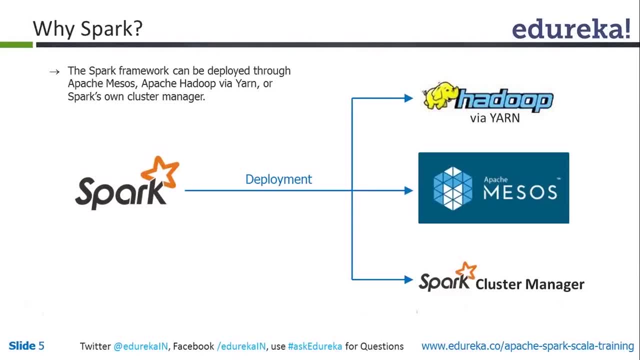 High level tools and many more things. there are some- some of the you know- other features which will come. so now coming to why spark? ok, so there are various reasons. I think one reason which is mentioned here in this slide doesn't really give you enough or see for. 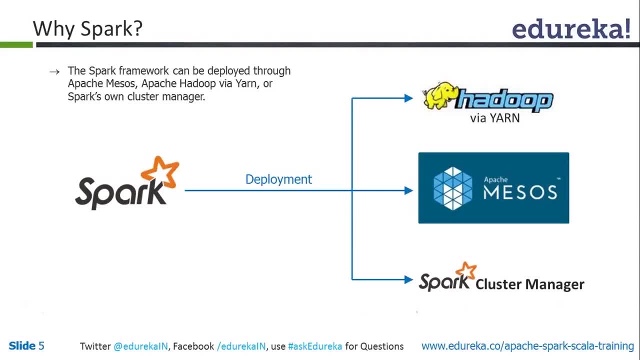 me, if I am going to spend my time and money to learn some something, I should have a reason behind it, right? so it is about why spark? this is one thing. but, guys, let me go off track a bit and it is kind of a deviation, but yes, it would help. see, you know, most of you would. 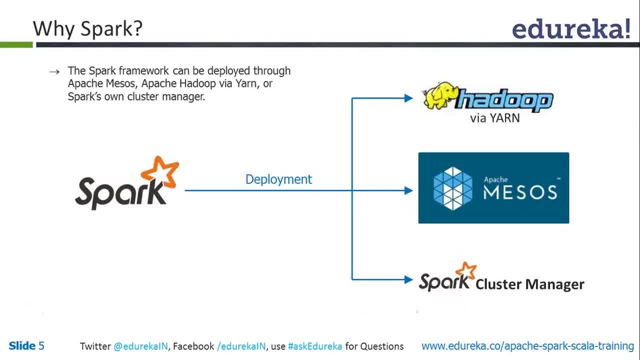 have heard about Hadoop. right, Hadoop is typically good for batch processing of huge amount of data, big data all together, and then it is quite flexible and so many things all together right Now why Hadoop has become so popular. initially it was not, of course. it has got some popularity. 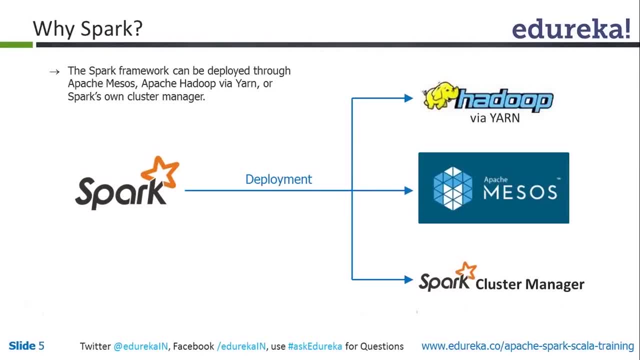 over the period of time. and also you must have got a clue when you were typing whether you have worked in big data or not, or probably some people who have worked in Hadoop or not. the reason is: Hadoop is a framework. Hadoop is not a specialized tool. what I mean by that is what is a framework framework provides. 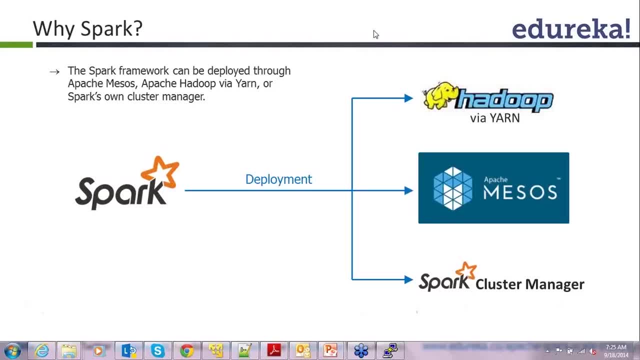 you various utilities or tools to do what you want to achieve. so, similarly, when it comes to Hadoop as such, it provides you various utilities to store the data. it provides you SDFS to calculate, to basically process the data. it provides you a paradigm called MapReduce. 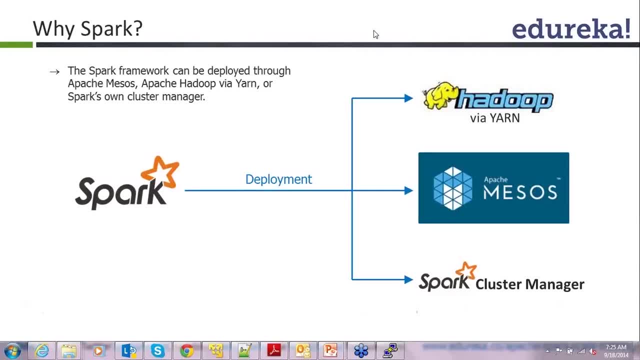 abort base. of course M2.0, it has change of it. but let's, let's just strict to the very basic 11 versions. all together right for the data ingestion, for the data exports. it provides you scooflume right copy from local, that plain, all copy from local for almost you know, SQL processing. 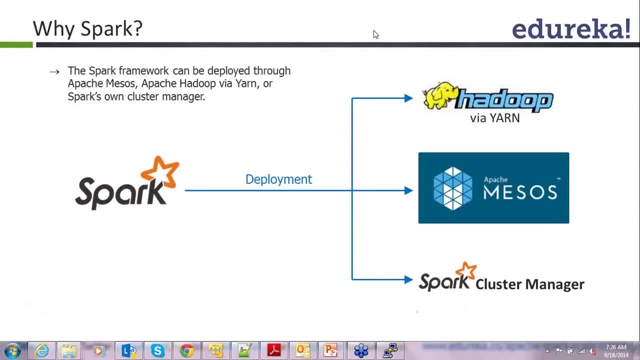 it provide you high right So for that. so the point which I am trying to prove is that you open your HDD file OR some SQLким. you can create any screendat When you have a screen객 which is talking about an command or command called PCI, maybe. 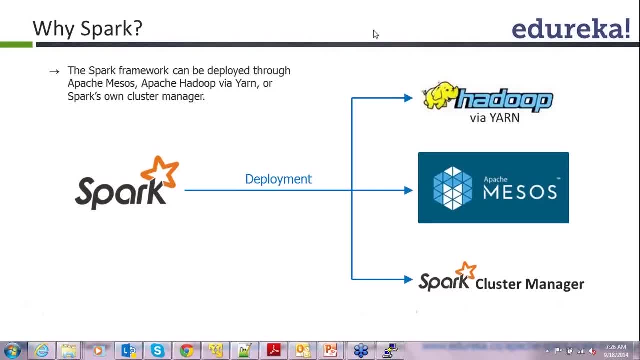 you have a particular kind of command, but essentially it is a very Nam-S eng singer. you are able to see, Hadoop has become so popular because it's a framework. it is not a specialized system. it is not that, hey guys. can you perform SQL queries on this huge amount of data? let's. 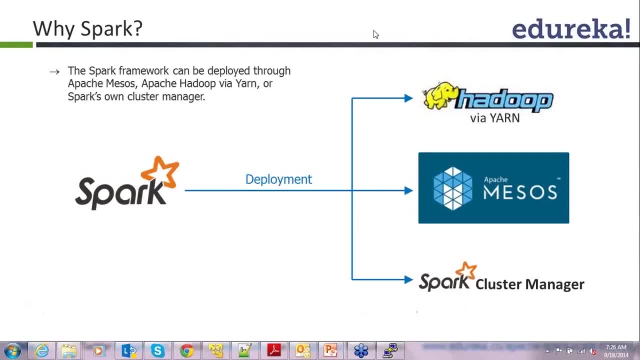 take this solution. no, it is a packet of all, or it's a bundle of all of those solutions built on the top of those two core components. right, and that's why it is popular. But then there are various specialized big data systems altogether. you must have heard. 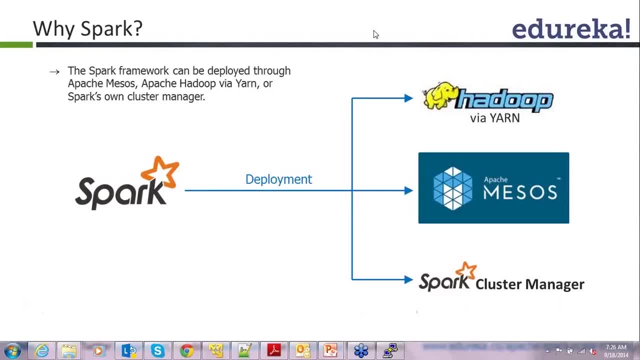 about Cassandra. Cassandra is a close cousin of HBase and nothing else. but yes, it has got certain advantages as well as some disadvantages. or you talk about Storm. Storm is. Storm used to be considered as a very close competitor of Spark, in fact before Spark. so when I 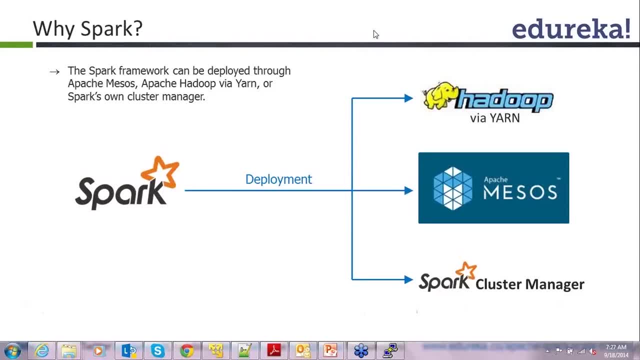 initiated this course of Storm at Edureka, we were quite excited. in fact, we went for one particular project, One particular project in production. now we are planning to move it to Spark. anyway, the point is Storm, again it's a fantastic system, but again it's a specialized big. 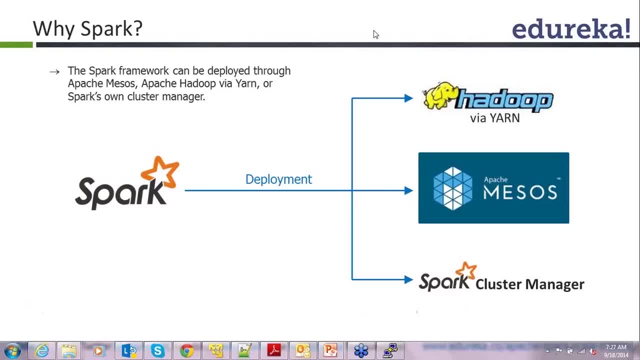 data system. it is typically used for the streamed data processing and nothing else. but then their biggest differentiator when it comes to Spark is it's not really a specialized big data system. you must have seen some of the glimpse earlier. you will see it in bit. 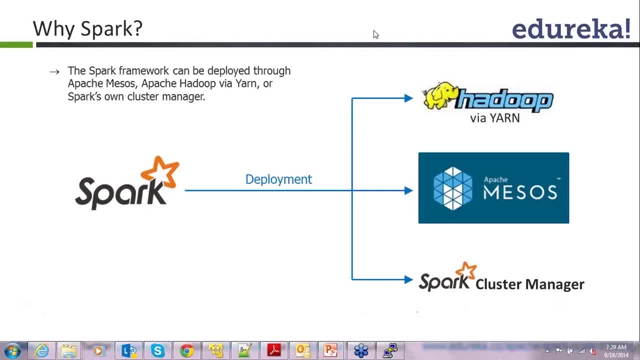 more detail in the future, In the coming slide, wherein you must have seen that we talked about Spark SQL, we talked about MLLiv, right? so what exactly are they? they are the different tools to do different things. you want to perform some sort of machine learning algorithms. you want to apply them. 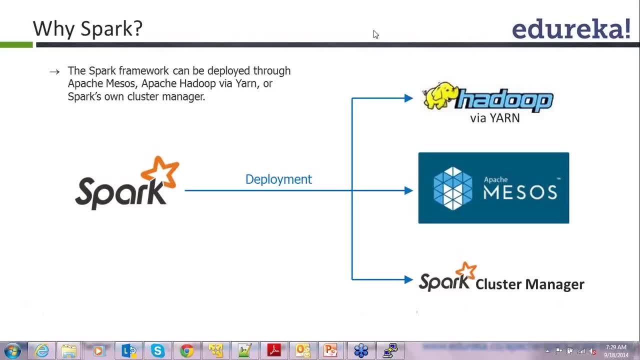 you have MLLiv. you want to do some sort of SQL analysis on kind of structured, huge volume of data. go for Spark SQL or Shark, for that matter. right, You want to do some sort of stream processing? go for something called Spark streaming. I'll. 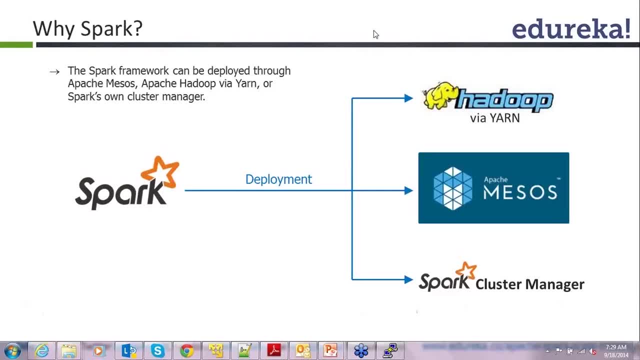 come to that very soon. So the biggest USP for Spark is: it is not a big, another big data or specialized big data system, it is actually a you know framework in itself. okay, In between there is a question. I'm not taking many questions, but there are kind of you. 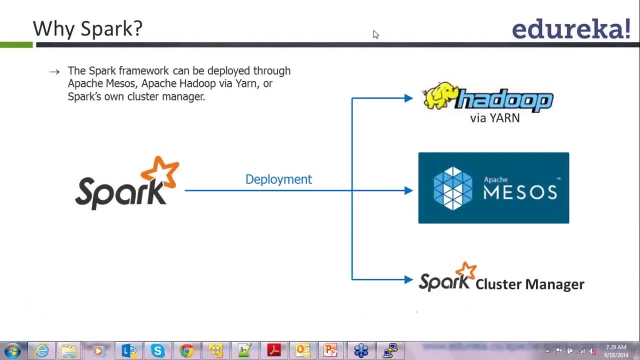 know this is a repeated question which is coming, and latest one is from Sharath. so for R language, Is there any support for R language? So let me just tell there is something called Spark, basically R, Spark or Spark R. okay, 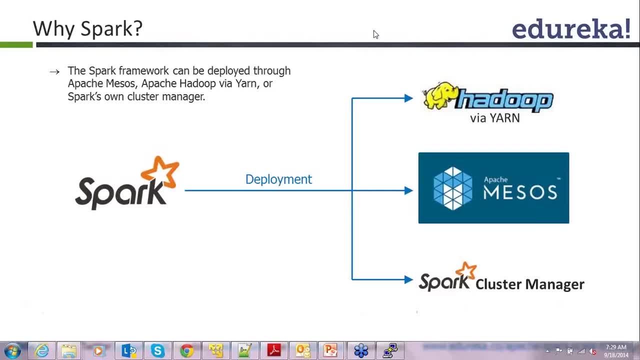 For now it is not even released, but it is still kind of WIP. okay, So, just like you have R Hadoop, etc. right? So, guys, definitely you can just type, you can type your questions. only thing is whether. 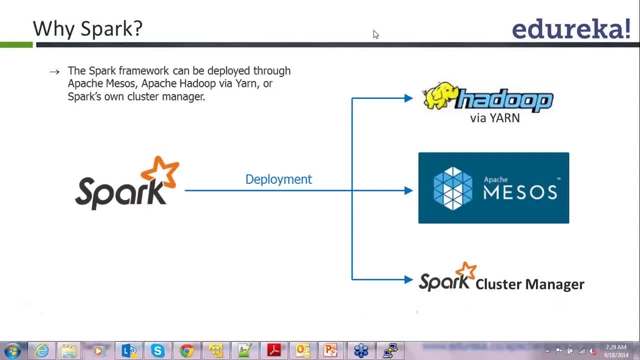 I would be able to answer them right away or not is a question. it's a different thing. okay, So if I'm not able to at the start, if I'm not able to answer them right away due to the time constraints and all we do have the Edureka you know handle, I will repeat that. 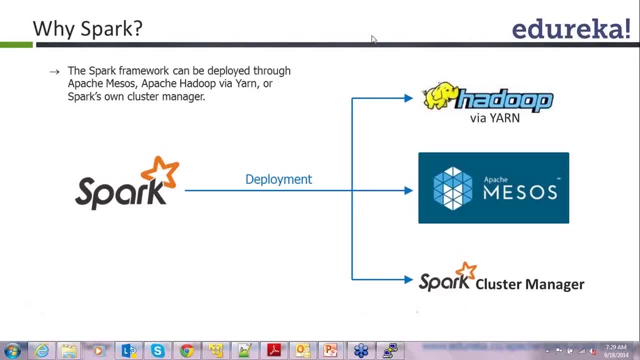 Edureka handle at the end wherein you can post your questions and you can get the answers. okay, I'm just kind of taking only very common questions, kind of right now. so that was the first USP. Now coming to the second one, it's about: it's not just. it is not just a freebie, it's. 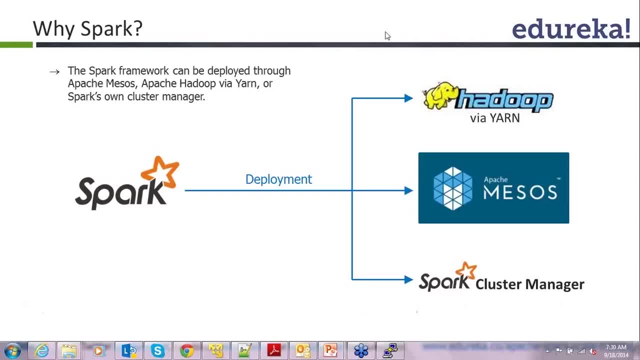 not just a freebie. it's not just a freebie, it's a freebie. it's a freebie. it's a freebie, okay. So that was the first one. It is. so when it comes to Spark Spark, you want to run it separately? you can run it. 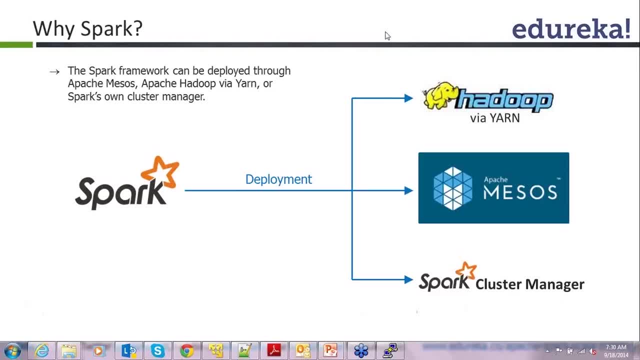 as a Spark, you know, using a Spark cluster manager, You can have its own. Spark has its own cluster manager, Spark cluster manager. It can run on a cluster of machines without having any Hadoop, without having anything. You want to take the advantage of Hadoop either from the storage side or from the processing. 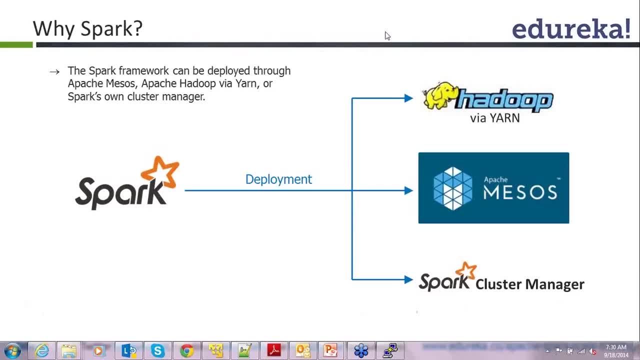 side. go ahead. You can integrate it with yarn and then Spark seamlessly integrates with yarn, though seamless is a very, you know, flashy term, of course, if you are talking about open source world. so there would be some nits and grits here and there, but still right, or you can have. 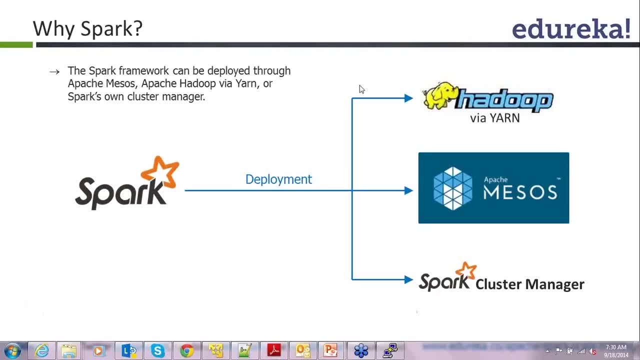 the under kind of, you know, cluster manager. It is quite popular but as of, in fact, neither I have used nor we are going to implement it within the course. Okay, So that integration of Spark with Apache Mesos- Apache Mesos is under cluster manager. 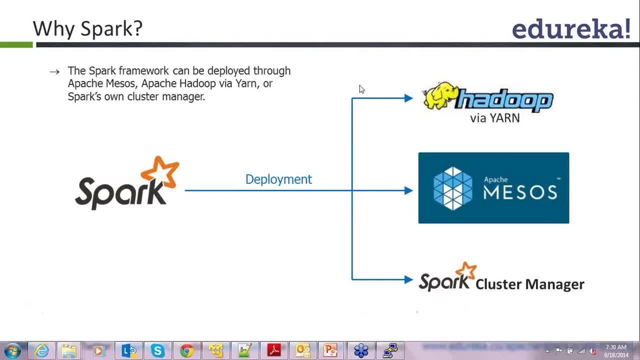 which you can, you know, use on, you know, basically as a. so it basically it is a cluster manager and it can be integrated with Spark. So in the course we definitely are, so by default Spark cluster manager anyway comes. 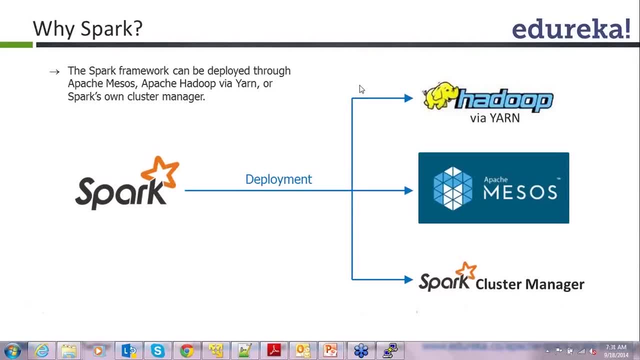 and we will be showing the integration with yarn as well. okay, In fact, last week only we completed it in the batch. Okay, So these are some of the good reasons. I would say not only so, this is not the only. 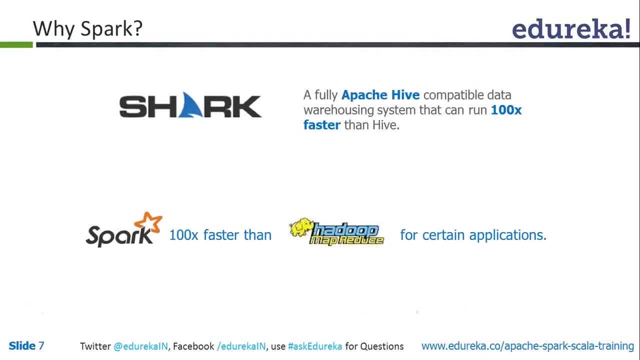 reason. other thing is: why Spark? again, this is more or less is the point which I have already covered- that Spark is polyglot. Right now there are three language supports: Java, Scala, Python and the focus for us. 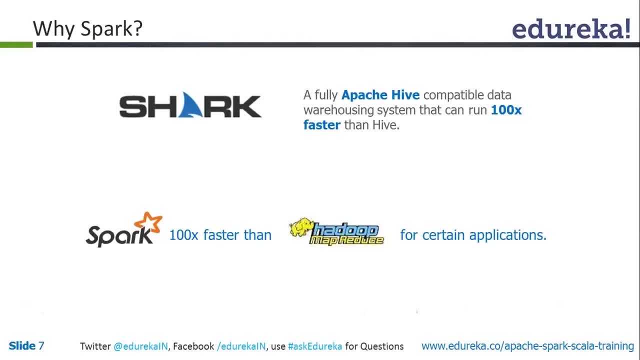 would be Scala. Why not Java or Python? I will come to that later. Okay Now, Just So. I was continuing the very same discussion of vice-part. so Spark, Now there is. I think I should have updated it. 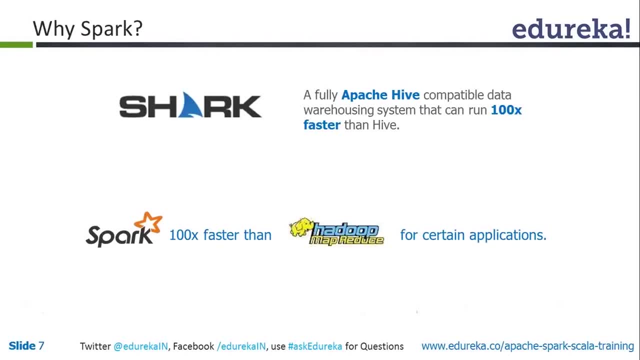 So by the time I started the batch, the first batch, and right now when I am taking this session, uh, Shark has closed. Okay, When I say Shark has closed, it doesn't mean that uh, it, it means that, uh, it is no. 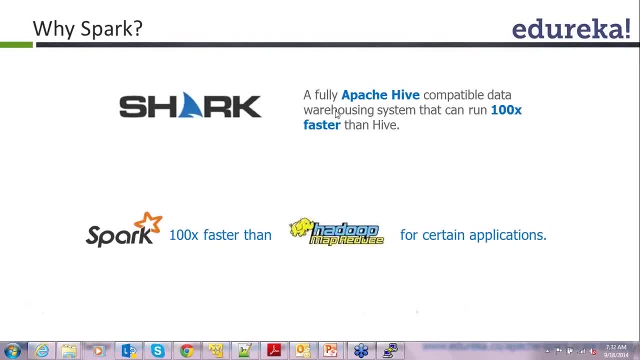 more valid. So What is Shark? What is Shark? Shark is equal to Hive plus Spark. Okay, So the entire reason for developing Shark was to integrate it with Hive so that those Hive queries, SQL queries and all which used to run very slow- I mean not slow, they were- 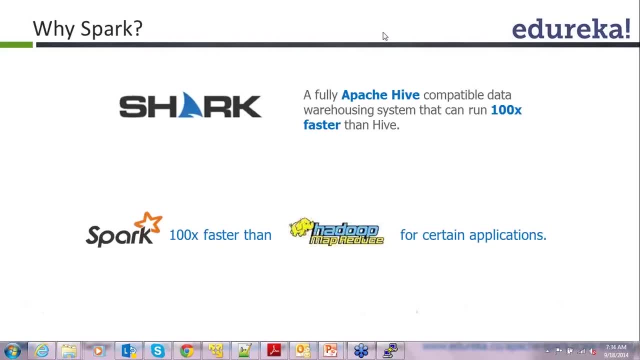 quite fast, but again for the medium set of data they were relatively slow. So So could we speed it up. That was the whole purpose. So Shark is equal to Hive plus Spark plus Hive. they typically call it as Shark. 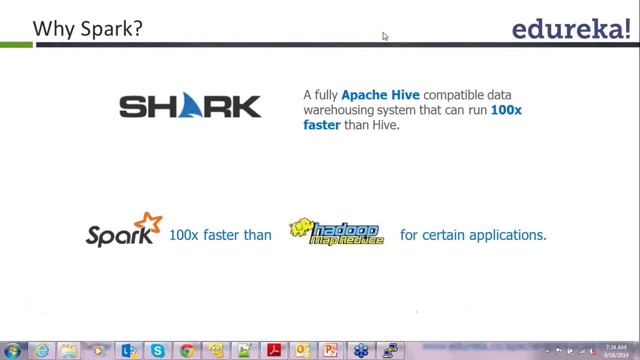 That was the project which was developed and it is quite popular as well. It is quite popular, but recently, not recently, probably some months back, but you know, uh, some months are recent. for us in Spark community it is kind of long time back. 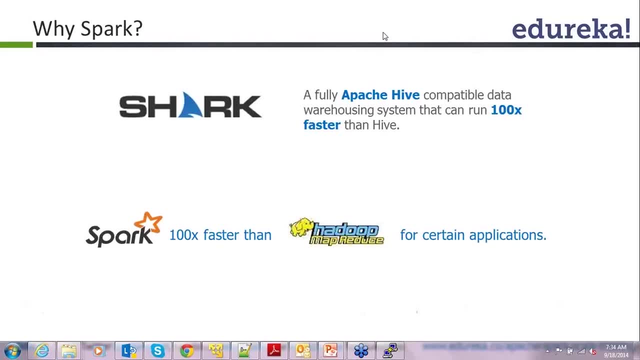 Okay, So, uh, uh, Spark has become a top-level Apache project. Uh, Earlier it was developed by Databricks and all and uh, now it has become a top-level Apache project. And then, uh, what they have done is there are some of the issues with, uh, you know. 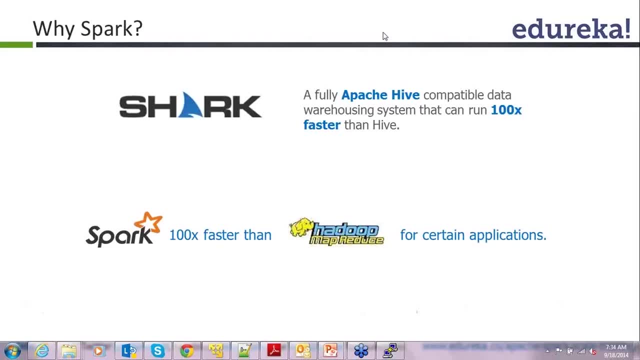 open source with Apache standards and whatever standards are followed for Shark. so they are changing their source code And the next release, or I would say Shark, will be succeeded by something called Spark SQL. So many of uh. if some of you have Googled or, you know, done some research on uh by 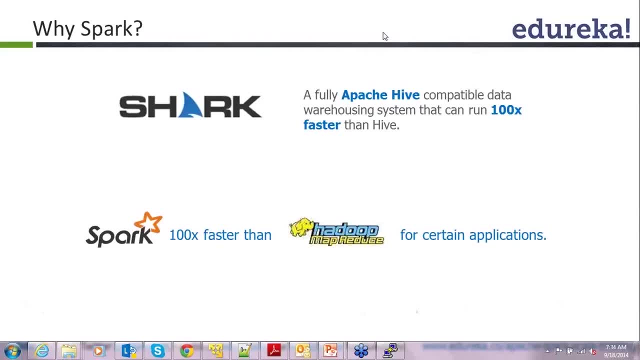 your own. you must have. you must be wondering: what is Shark? what is Spark SQL? So Spark SQL is going to. it's basically the successor of Shark and nothing else Right now. so Databricks and Apache have said they are going to stop it, so there. 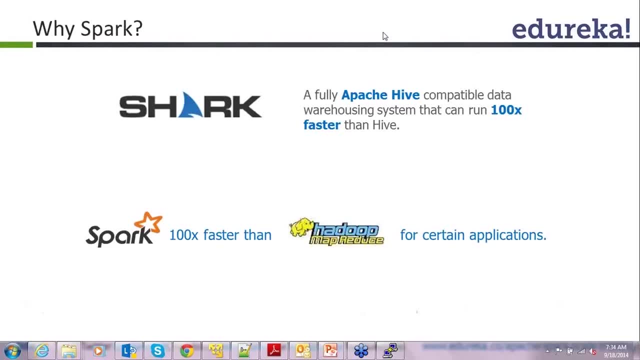 is no further development which is happening, but the support for current Shark is provided. The reason: Because Spark SQL is not available. Okay, Spark SQL is right now not integrated with Hype. Spark SQL using Spark SQL. probably. you want to read some JSON data. you want to read some. 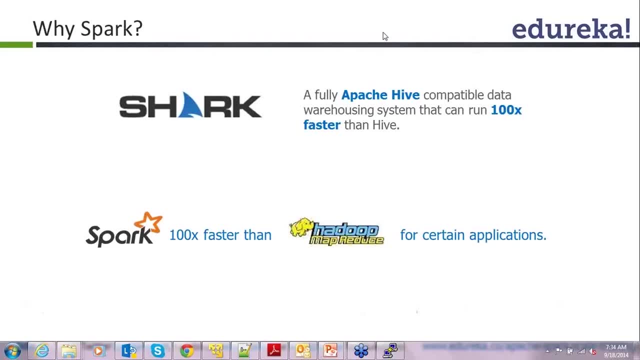 sort of uh, let's say, uh, you know plain text files and all in the form of some tables. you can do that, But right now it is WIP kind of So till the time Hype is integrated with Spark SQL, it is, you know, Shark is going. 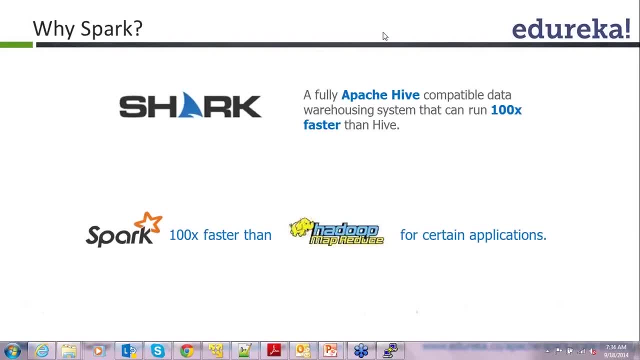 to continue for some time and after that you will see that you know the GitHub repository for Shark would be closed. Got it guys. But anyway, coming to the point that Shark- yes, you talk about Hype queries it makes, 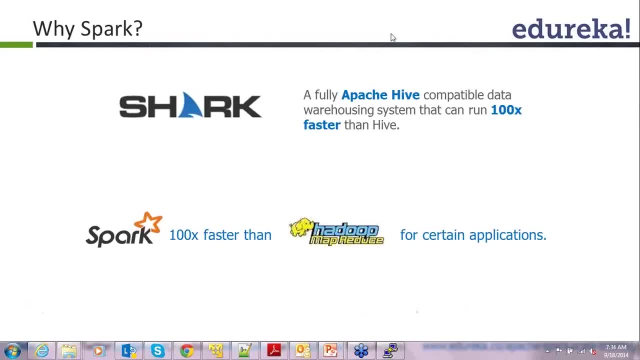 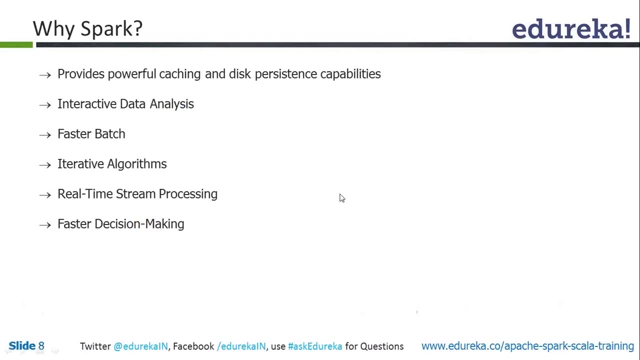 them. in some cases it is almost 100 times faster. You will see some, some example today, all as well. Okay, For some certain applications, Spark is definitely. you know, we have seen, I personally have seen Spark is almost 100 times faster, uh, than the Hadoop MapReduce application altogether. 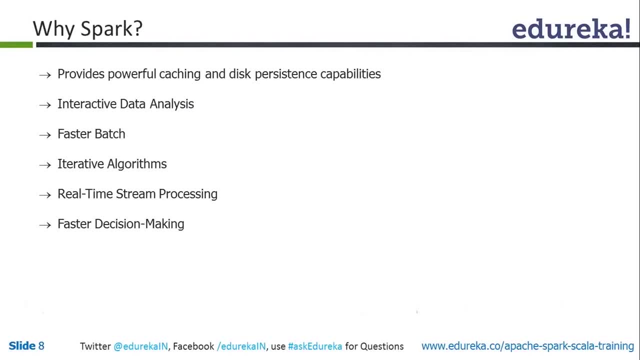 Okay, So, just to summarize: Okay, So, why is it? uh, so, why Spark? right? Uh, it provides you powerful caching and disk persistence capabilities. Powerful caching, caching- I'm sure you are able to correlate it with that: in-memory applications. 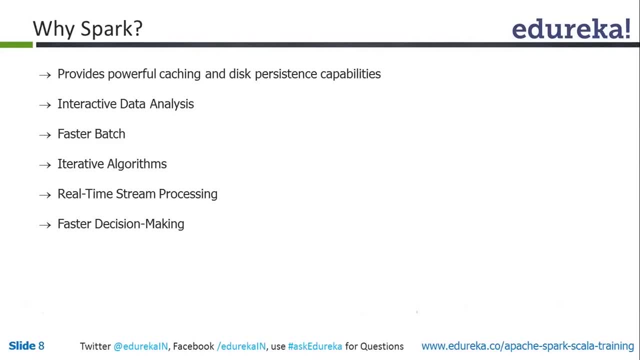 and all, And then disk persistence capabilities: right, So it can persist in the disk as well. Okay, It allows you for the interactive data analysis. Now when, when you go to uh Hadoop and all you typically talk about, you know you. 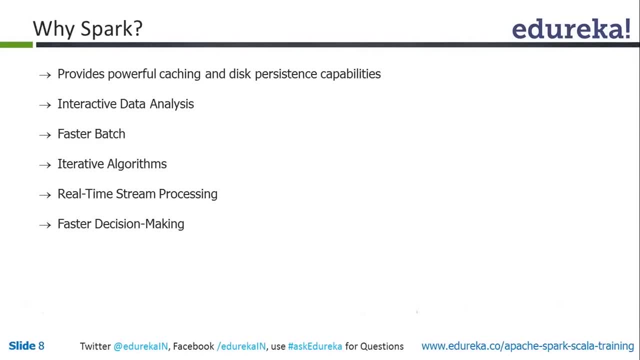 have to submit a batch and till the batch is done, uh is over. you never know what exactly is going to be the result. right, It's kind of a black box processing which is happening in front of you. But here, so it would. it is always good to have some sort of interactive data analysis. 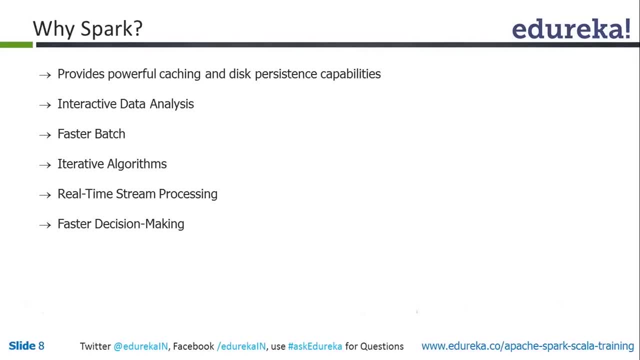 altogether right. Using Spark Core Engine, it is, uh, quite possible. Okay, Then your faster batch, again something which is already known. Now There are certain kind of you know algorithms which you cannot really implement in MapReduce. 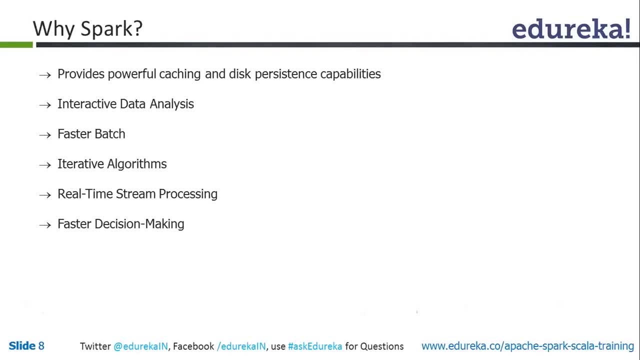 Talk about recursion, right. If I ask you to implement a Fibonacci series, you will not be able to implement it right. The reason is because it's a recursive kind of an algorithm. altogether. There are several- uh, several- asynchronous algorithms, iterative algorithms. 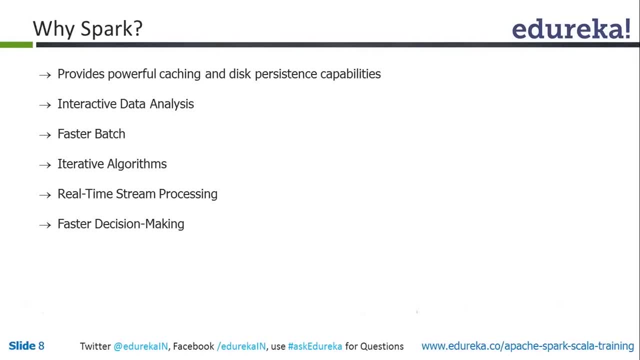 They're not really possible to. you know, do in-demand Okay In MapReduce world. But yes, you can achieve them in Spark. I'm not saying Spark is going to support all of the other algorithms also There are. it has also got its. you know usual limitations of the distributed systems. 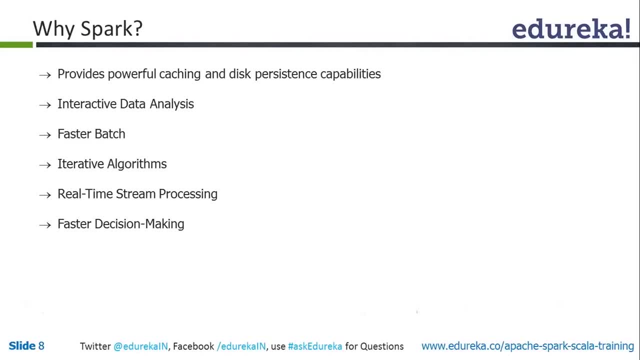 But, yes, uh, many of them are quite possible. Okay, Uh, real-time stream processing. This is where, uh, you know, Spark has that, has got that knocking power over. uh Storm, Wherein Storm? here Spark becomes a super-power. 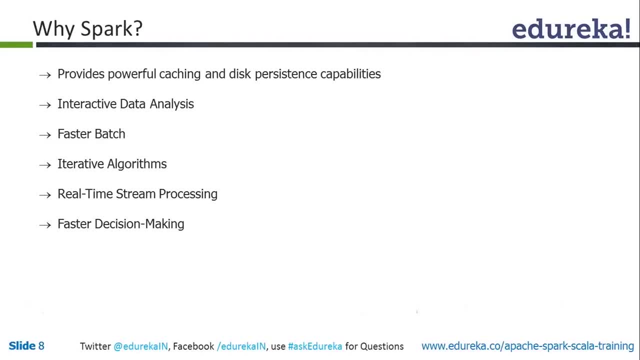 Super set of Storm, Or rather than I would go opposite way. Storm becomes a special use case of Spark Okay, Wherein it typically leads to this real-time- uh, you know- stream processing altogether, And of course all of that typically leads for the faster decision making. 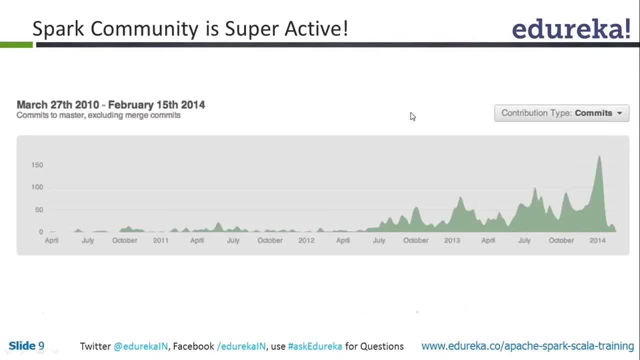 Okay. So these are some of the reasons, uh, why Spark basically Okay Other thing, Okay Other thing- is about your community. So Spark community is something Okay, This is something which is super active. You can actually see that. 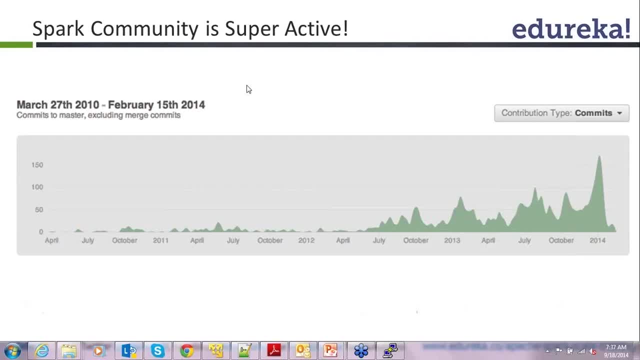 This is, uh, something which we have not produced. It is, uh, typically, uh, straight out of the GitHub repository: commit, So it it just tells you how many commits have happened. If you see October 2011 and all they have been, basically, by the time it was you know. 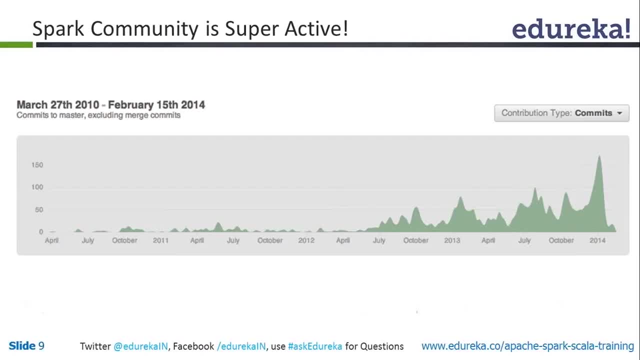 kind of being formalized And only a handful of the developers were working Around 2012,. again, there was hardly anything. Then, all of a sudden, around 2013, and right now It's about 2014.. You can actually see what exactly is the overall, you know, commit rate, which which is coming. 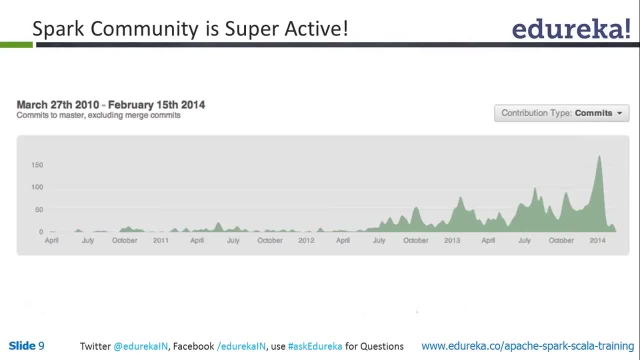 up, Right? So this, this community, is quite active, And when it is quite active it looks good. but uh, you know you are all developers as well, Right? Or probably you know some senior people. You must have seen all of that. 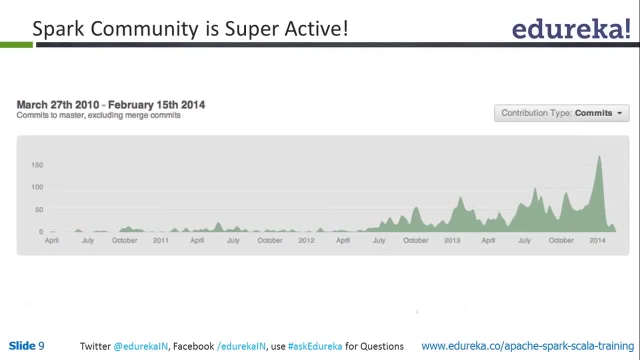 When you talk about super active, Of course, Right now The system is also a bit turbulent. When I say turbulent, it's like uh, every release something or else would start, you know, uh kind of working, or there would be some of the features, of course, which would 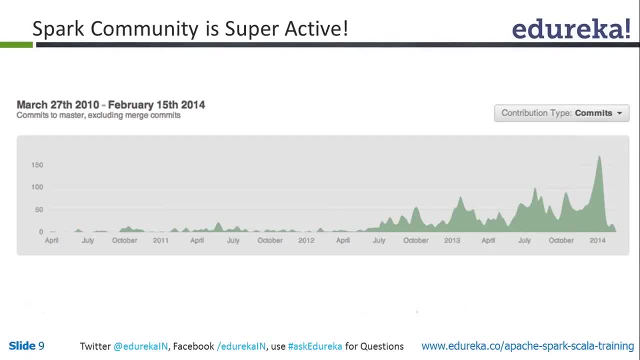 not be working so well. they are right now fixing it up, But we are hoping that you know very soon it- all of that would be stabilized, kind of thing. Wait So To tell more about Spark. uh, from the good things. 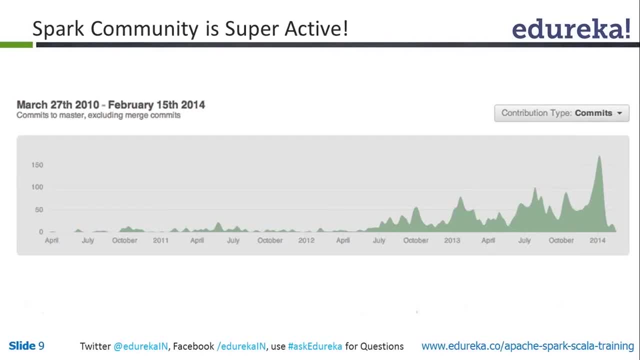 But you should always see what exactly is right also Right. So, uh, the recent uh release of Spark there has. there is some problem in Spark SQL right now, which will be very soon, I think it will be fixed, kind of you know, within a week. they gonna fix it as well. 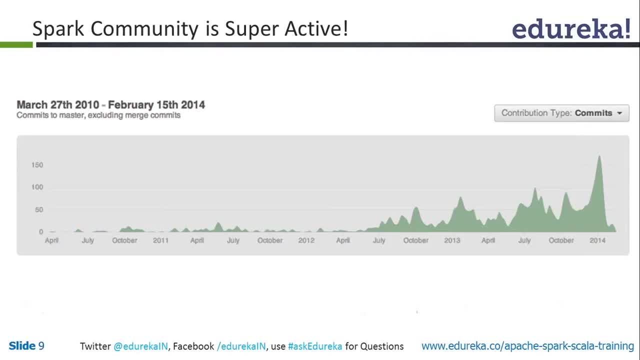 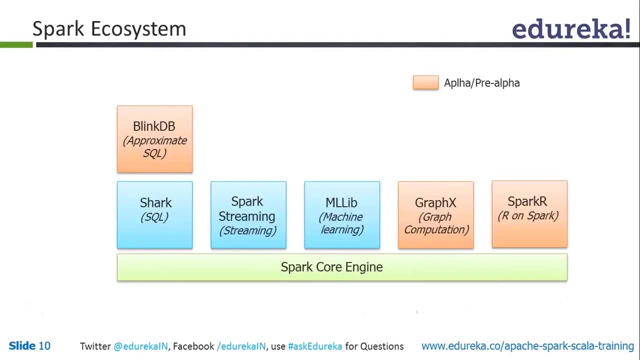 So they always tell when. when a specific version becomes a stable, they say that, okay, now this is something which is uh, good to download, Okay, So, But anyway. So the idea was to tell you that, yes, it, this community is quite active altogether. 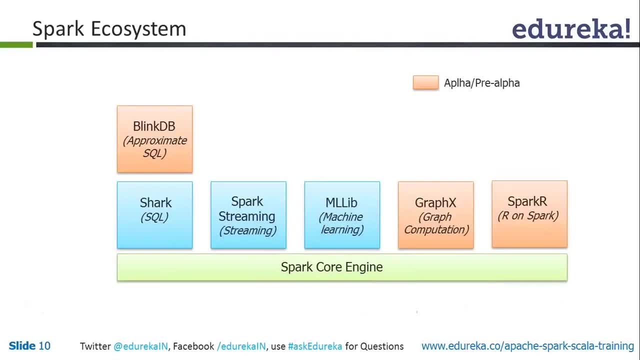 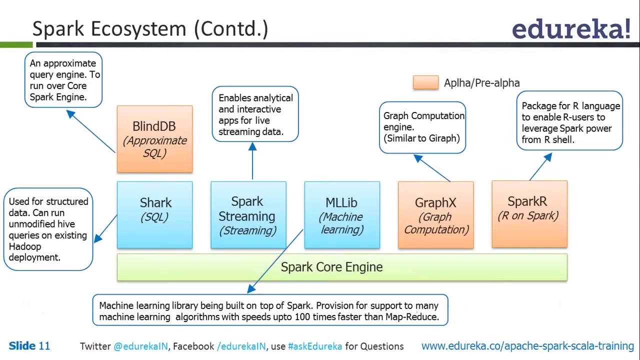 Now this is something which I was talking about sometime back- that Spark ecosystem. Spark is something which is not a specialized system altogether, So it is a framework, and that's what we mean by a framework. right, That's what we mean by a framework that you can actually see here, that at the bottom of 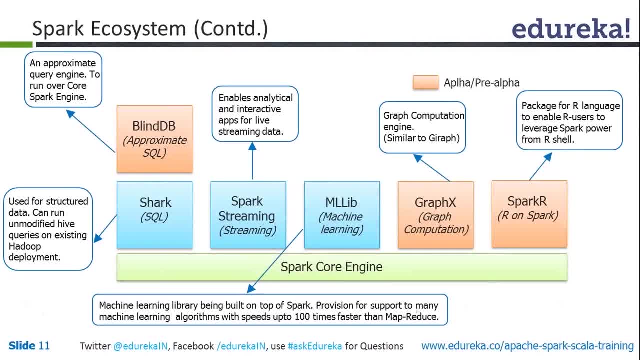 it. you are having, typically, just like any framework, You should have a core engine right, Hadoop, You have a core engine. You have two core components: from the storage side- SDFS- from the processing side- MapReduce. Similarly here as well, you are going to have a Spark core engine and then you are having 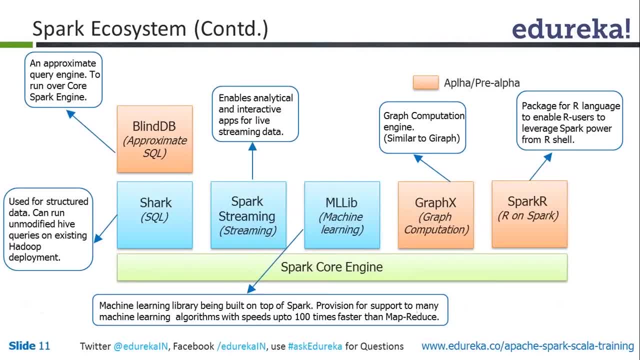 multiple wrappers. on the top of it You have shark. I would say shark slash, Spark SQL. Okay, Just to correct it. I hope you are able to correlate right. So shark or Spark SQL, Spark streaming MLM graphics, Spark R- probably somebody was asking. 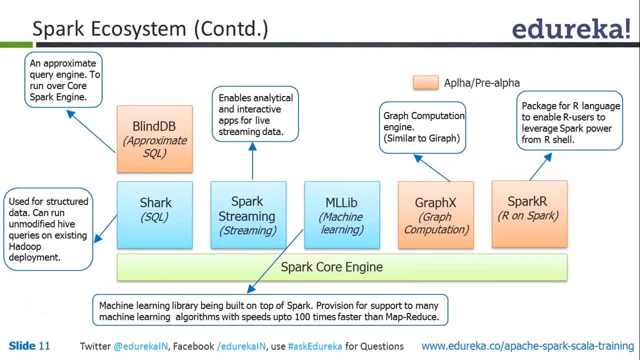 about Spark with R. It is not yet released. So you can see that this orange color thing. they are still on alpha or pre-alpha release. Okay, Blink DB, approximate SQL- Okay. So now what exactly they are? Let me just give you a brief hint about them. 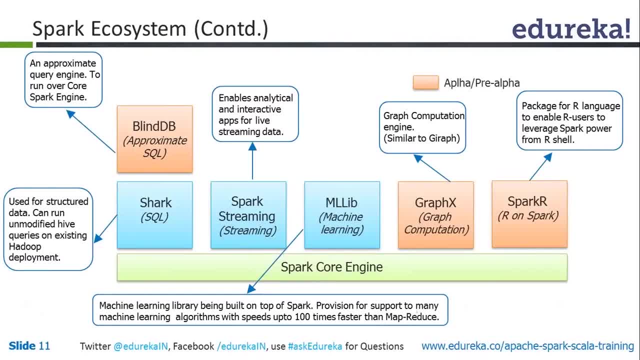 Okay, And then let me tell you some more things which are kind of you know, which you should expect in coming future altogether. Okay, So come to shark. I think I have already told you You have to do, let's say, some sort of you know, SQL analysis on the structured data. 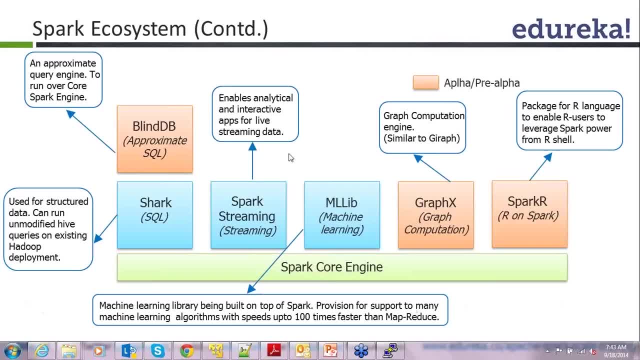 in a very fast manner. Shark is your answer. You want to perform some analysis on the data which is coming. Okay, You want to perform some analysis on the data which is coming in the form of streams. Now, this live streaming data might be any data which might be coming from you know. 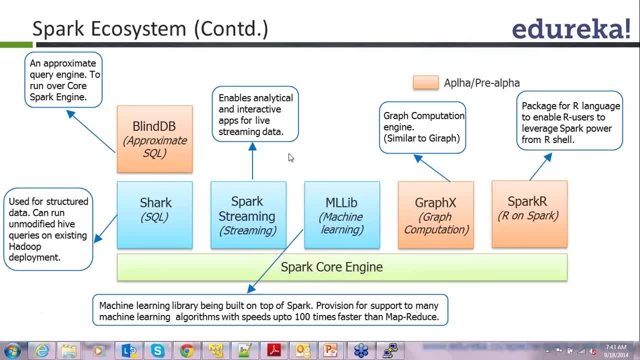 those distributed messaging systems like Kafka, zero, MQ, et cetera, et cetera. or probably you just want to create some sort of file watching capabilities, but in, as in when there is any data which is returned to a file or to a directory, you should be able to do. 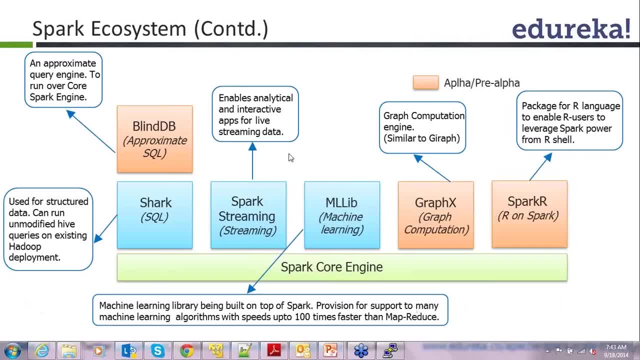 something right. So they are typically do the streaming kind of operations. Yes, You can perform all of them using something called Spark streaming. Then machine learning, ML live. ML live is something which is, again, it is a machine learning libraries which is, you know, which is based on the top of Spark. 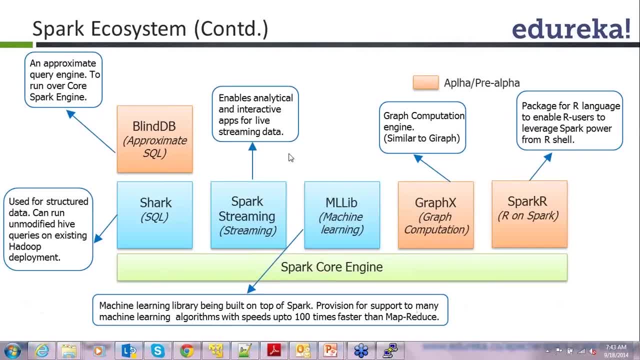 And, of course, the biggest advantage which you get is your typical machine learning algorithms. So what is the machine learning library for Hadoop? It is called Mahout, right, And Mahout is quite good, But again, Okay, So ML live can perform the very same machine learning algorithm or can implement the very. 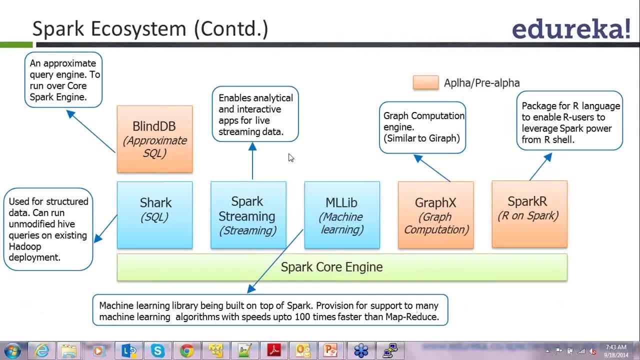 same machine learning algorithm, almost hundred times faster than Hadoop, In fact, as an inside information or whatever that you can, the next, next version of Mahout they are. I don't know next when it would be released, but the next thing what they. 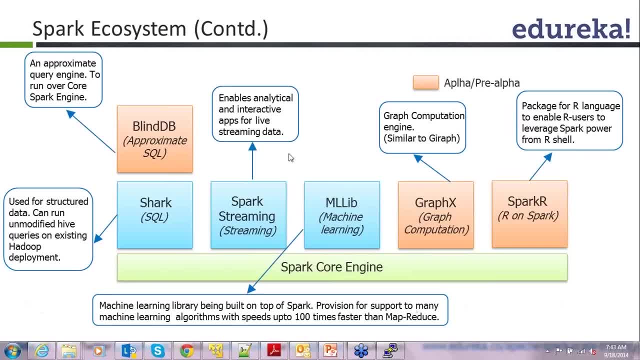 are trying to do is they are trying to port entire Mahout functionality into Hadoop- Okay, Okay. So you get ML in the assembly does not have the same functionality into ML live. Of course, everybody wants to take more power, right? So ML live is something which has evolved. 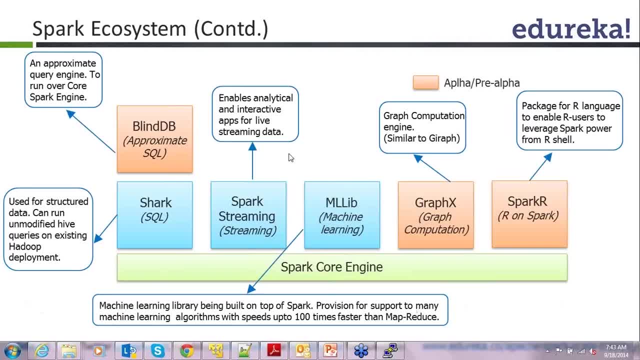 It has got some, uh, machine learning algorithms available, not some, quite a few, I would say Uh, but still it is not yet that much enriched, as Mahout is right, Because you can easily see that, I mean if you see the release rates and all they are. 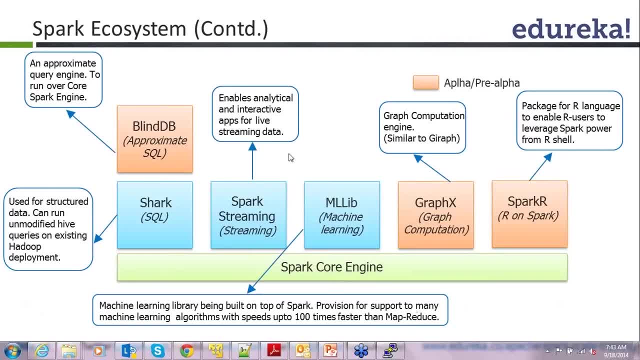 hardly some one year back, Whereas Mahout and all are since last summer, Okay, almost four years plus, right? So just they are maturing over the period of time, but at the same time they are becoming much better, right? Talk about graph computation all together. 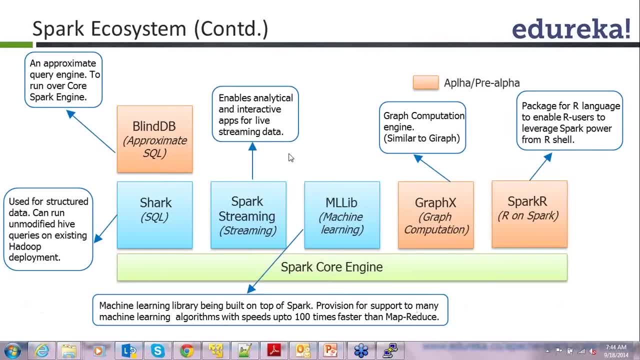 so you must have seen Neo4j, JRAF graph lab, etcetera, etcetera. So typically it is in the. so again it spark gives you the utility to perform your distributed processing all together right, distributed graph processing. 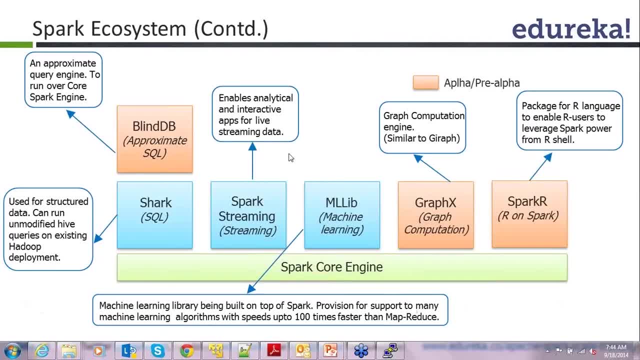 Not related thing, but yes, before graphics it used to be called as bagel. ok, So bagel it was. I mean, just one year ago it was released as bagel. then it got changed to: I mean it will be succeeded by graphics in the again, it is in the transition phase right now And 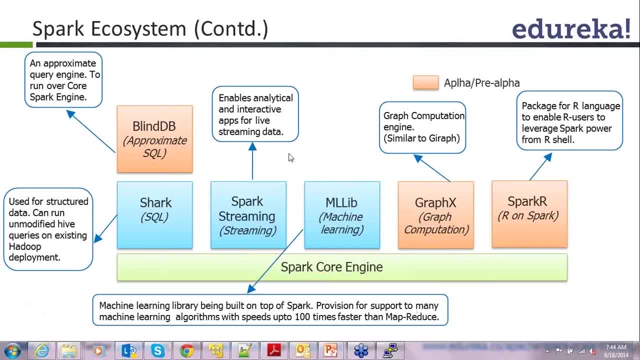 spark R. I think I just told about it. just like R Hadoop people who are from R background they were. They want to utilize the power of Hadoop right. they typically go for R Hadoop and which is typically by revolutionary takes, and now they have the. you know this thing with cloud era. 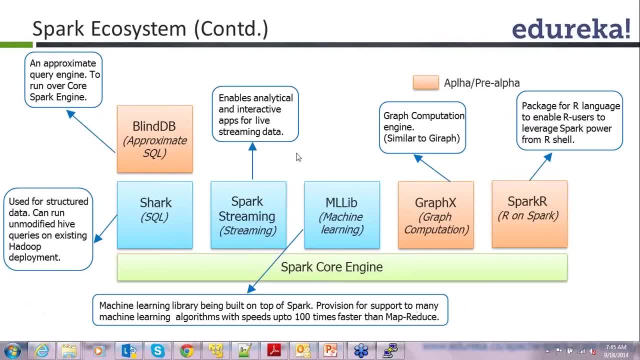 but yes, that is in the Hadoop world. You talk about spark with R, spark R, is your answer right? So these are some of the things which are coming up. in fact, what I heard latest was that, just on the lines of hive. 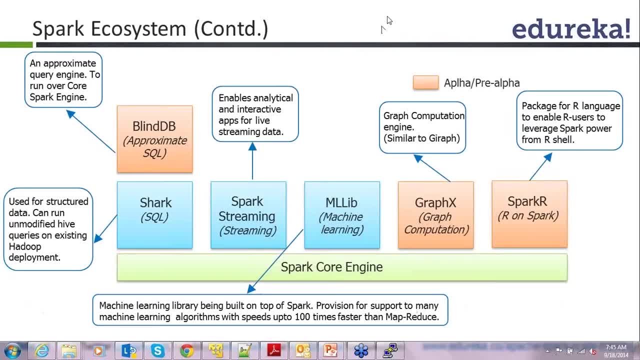 People want to move pig also, pig right to spark itself and, if I am correct, as of now, they are calling this project as spark S P O R K spark. ok, When it will be released, when it would not be, I do not know about that, frankly, but yes, it is kind of, you know a. 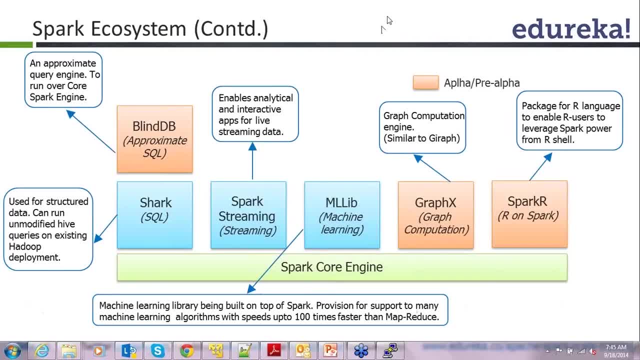 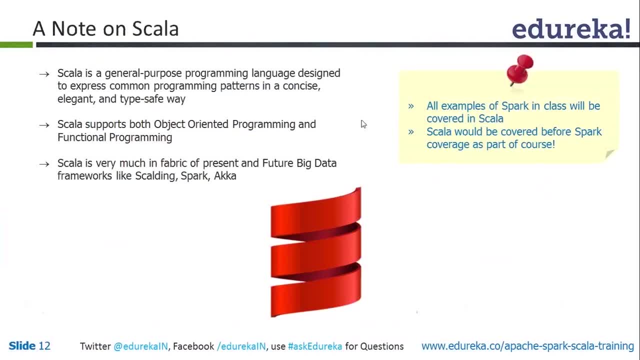 project which is already going on right now in Apache. So you should hear something about it, right? So, anyway, That was just to give you an idea that, yes, this ecosystem is something which is just enriching over the period of time. So, guys, how are we? Are we good? Because we are almost. 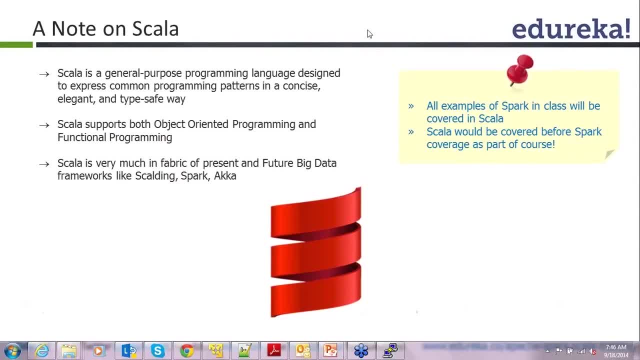 you know three quarters of our entire time. Was it useful for you? I am now, because I am now moving to the next, that section of it, right? I hope it has added some information to your existing repository. all together, that was my purpose, right? Is there anything in? 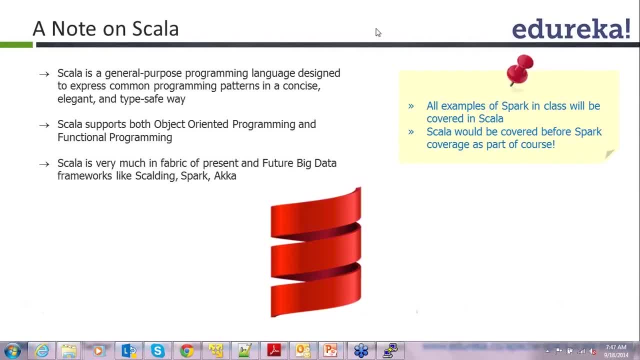 the lines of his base, actually, that nothing is required on the lines of HBase because it so you can. you can think about Blink basically. no, actually you do not really have anything in the lines of HBase. actually you do not even require. with Spark, You will realize. 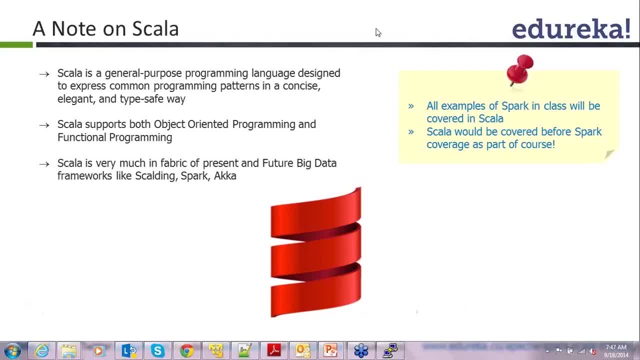 it. this is- I would say this question would not be valid when you will learn what exactly is the use case of, you know, spark. okay, satish spark is something we will take over to hadoop. no, no, no, no, no, no. so many people who are asking this question that it means spark is going to- uh, you know. 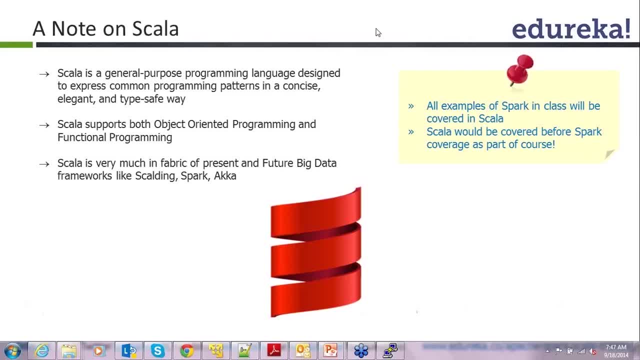 uh is going to take over, hadoop, going to replace it? no, guys, that's why i, at the very start, i told, or i requested to, to, kind of you know, search for something called, uh, lambda architecture. okay, that would give you more idea about how exactly they are going to coexist. 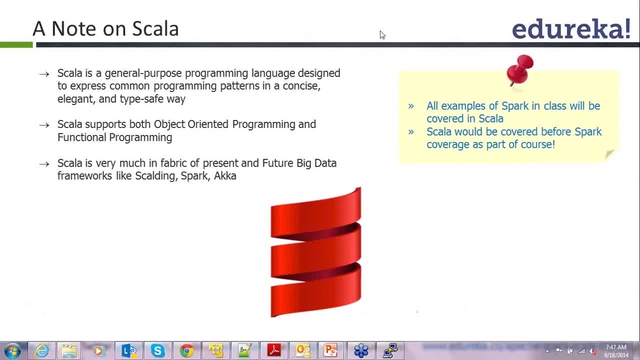 and how exactly they are going to complement each other, right? so just an answer to most of you people, right? okay, uh, somebody is asking about the question about what exactly is map reduce equivalent in spark. so, guys, uh, actually i'll move to this question, uh, now, so nobody has asked me. 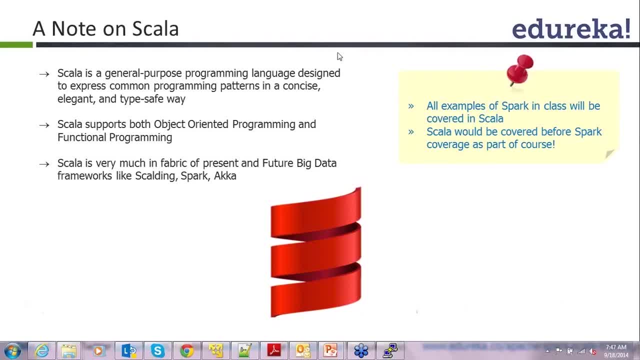 this question? uh, okay, and i am going to answer that in a few more minutes. okay, now a note about scala. so, guys, again, scala is just like any other programming language, yes, but yes, it is typically called as improved java. okay, and it's a general purpose programming language altogether, but when? 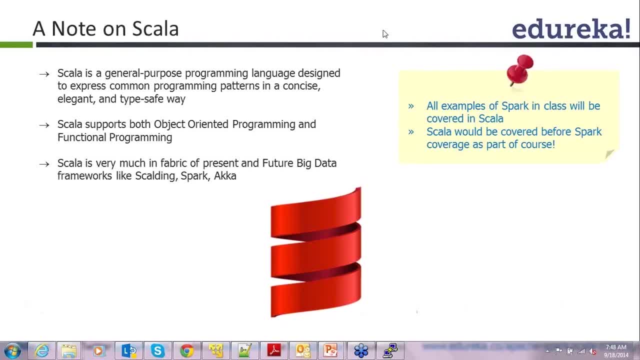 why are we calling as? why are we calling it as improved java? look at the second, second uh point. scala supports both object oriented programming as well as a functional programming paradigm altogether. that's the biggest advantage which you get with scala, because you talk about typically those distributed processing systems altogether. then you don't really code in the 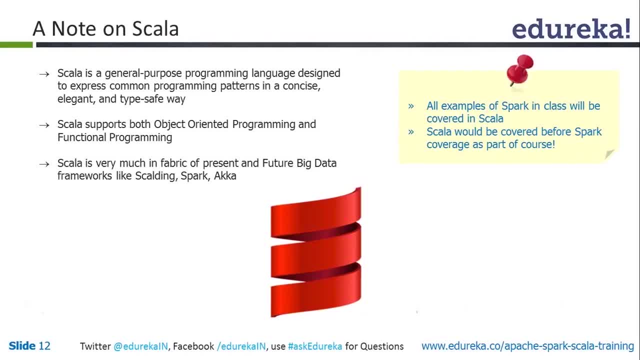 object oriented way. you must have seen it. you must have observed it in the terms of map, reduce programs. if you have written earlier, you must have seen those kind of design patterns which come along with it. you don't really i mean, applying object oriented programming concepts is not really. 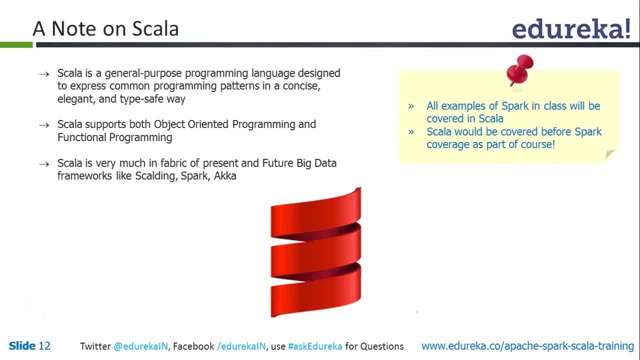 a very good way to you know, implement them, so that that is one of the main reasons. you know it lags, though, for underlying framework is written in java for where, where, exactly where you need those classes and those those kind of, you know, uh, object oriented programming concepts altogether. 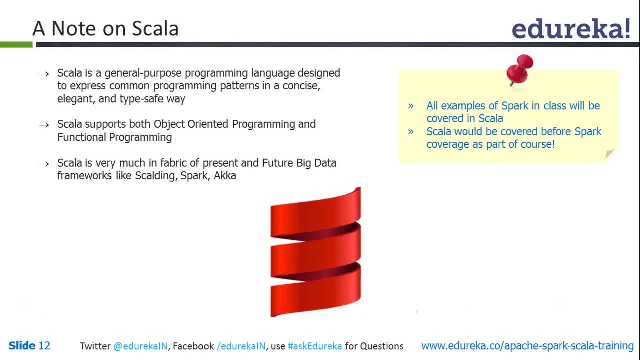 but when it comes to the maverick's kind of applications or most of the distributed applications and all typically, people have found that functional programming is something which is quite good. it's not really the object oriented programming. and then there are other aspects which come from. 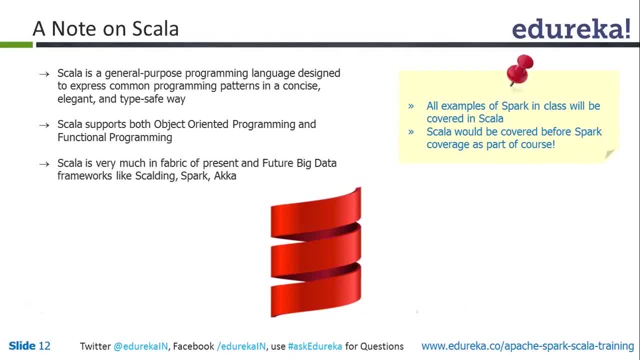 the concurrent access, and then it becomes very, very difficult to manage the concurrent objects, and all in the, you know, object oriented programming world, wherein you can change the state of something, whereas when you go to the function programming, since you have the basic. so what exactly are the two paradigms? 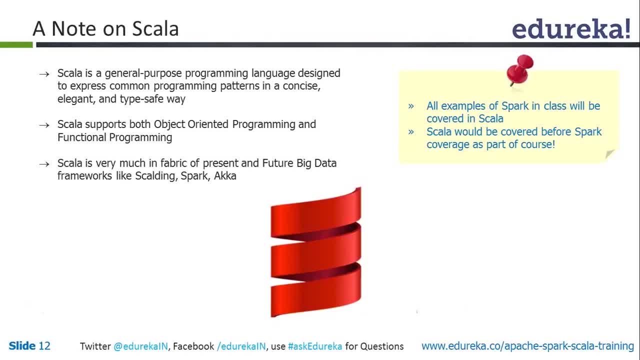 of functional programming. what exactly are the two main paradigms of function programming, guys? i mean, i'm not asking, it's not mandatory to answer it, but if somebody knows, you can just type it. so there are the two fundamentals. are that your functions? okay, your functions are the first. 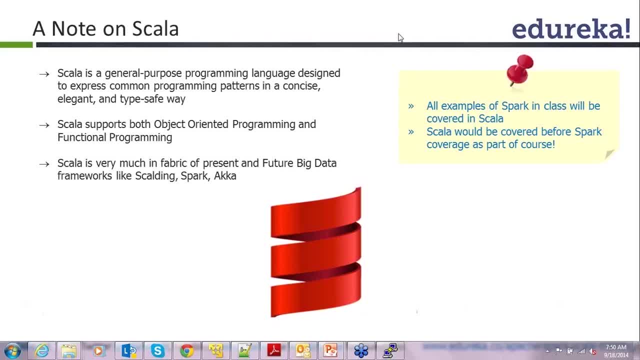 class citizens. when you talk about first class citizens, you will be treating your functions just like, uh, any variable all together and the other, uh other one is entire objects are immutable. so, uh, you know, it's almost kind of string. so if you change something you are not going to change. 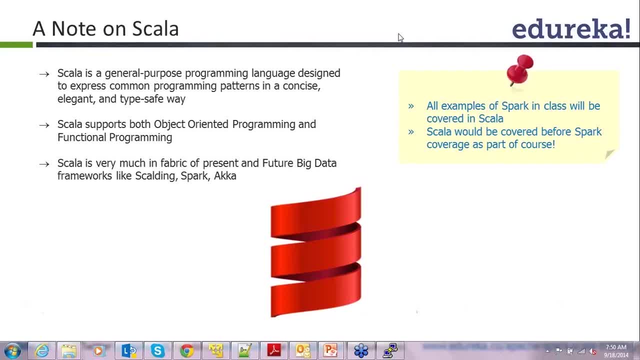 the object per se. you are not going to change the state of the object per se. you are going to create a new object and that, you know, immensely simplifies the problem of, you know, concurrent programming altogether. anyway, that's a separate topic. sorry, i sometimes kind of, you know, deviate a bit, but yes, it is about so with Scala the good thing is. 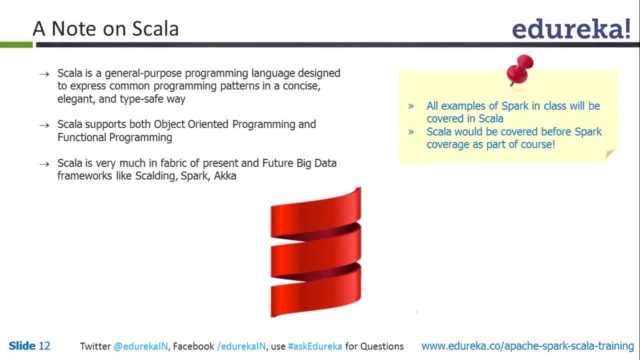 it supports both kind of paradigms all together and it is not that we are just, you know, going to learn Scala only for it, only for the sake of this course. no, guys, It is very much in the fabric of you know most of the future. you talk about future. 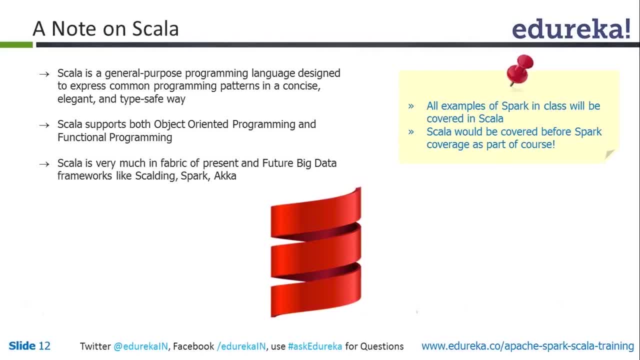 big data frameworks all together or some of the existing ones, Scalding. how about Spark, which you are going to learn, or some of you who will subscribe to it, right? or Akka is another one, right, it is actor based, multi actor based kind of framework and all. 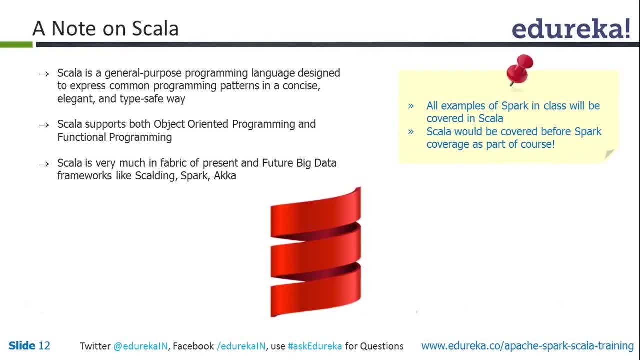 So they are. typically, all of these frameworks are completely into, you know, written into Scala. So, of course, all of the example- this note is also important- that all of the examples in the class will be covered In Scala, and we know, we do know, that most of you would not be coming from that background. 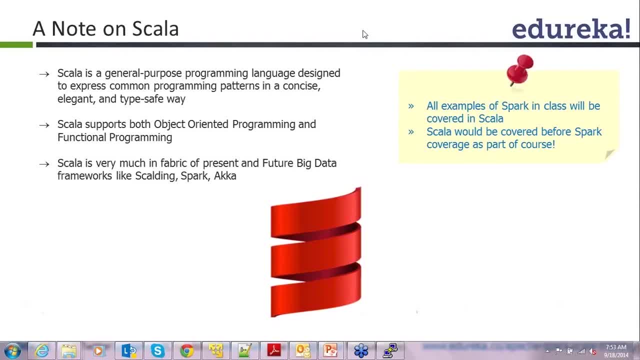 So, of course, how exactly we have defined this course is that first four classes would be focusing on Spark- sorry, Scala- to give you good enough information about how, to, you know, use it for the programming, the bare essentials which you need to know. Of course, we will not be telling you what is for loop, what is for while loop and all. 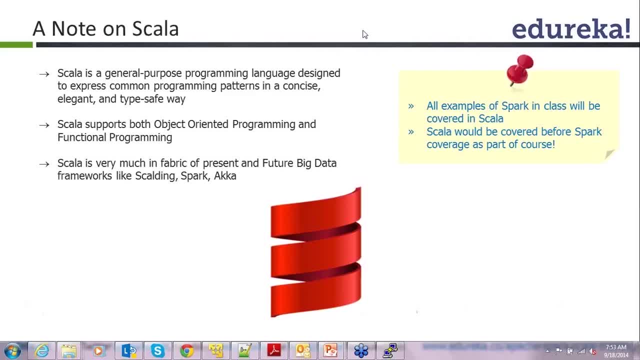 right, Because that is something which you know already. What we will be telling is how exactly they are going to be different in Scala from, let's say, any other programming language or, let's say, from Java. all together, right. So in the previous batch, I always have taken those parallels from Java. okay, this is how. 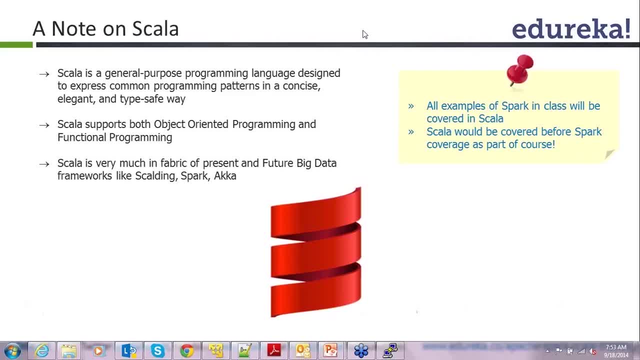 you typically do it in Java, but then, when you come to Scala world, this is how it goes. you know different. all together, right? So that's the overall plan here. okay, Now I will come back to the question, that question which was asked to me earlier, that 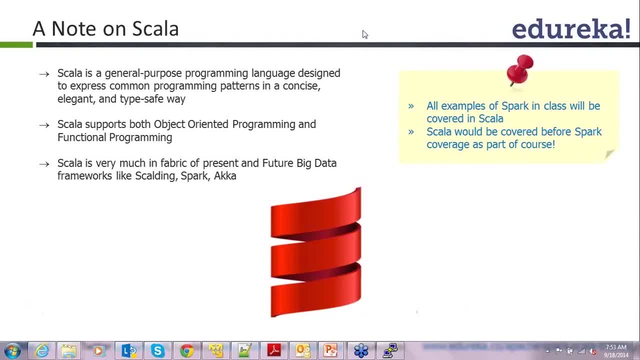 what exactly is the MapReduce equivalent in Spark? So with Spark you generalize your MapReduce program when we talk about MapReduce, so there is something called dot Map, dot Reduce. these are some of the inbuilt functions which are provided by something called RDDs, and all okay. they are the. you can treat them as Scala. 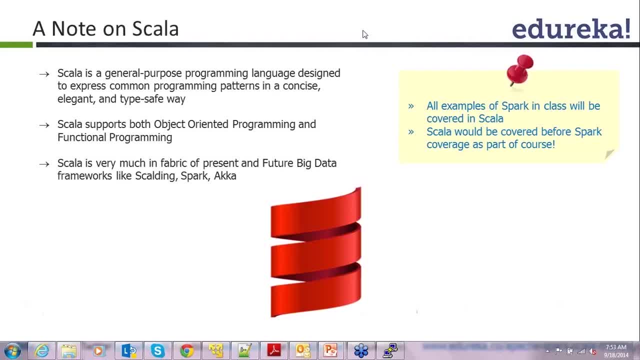 data structures all together. Okay, So you can perform them with the Map. you know, Map phase, Reduce phase, you can do all of that. okay, So they are just the functions which are provided by the RDDs. is that clear, Siddiqui Shijat. 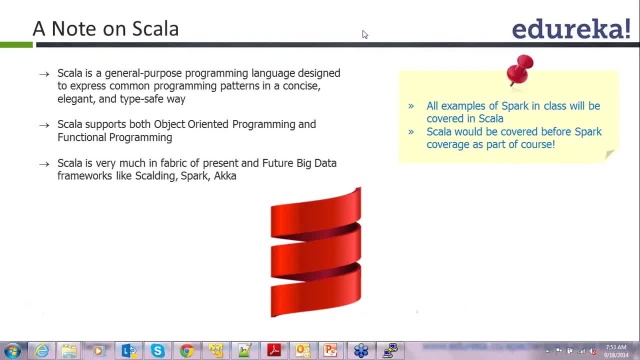 Siddiqui, that exact question was by you, right? And then the good thing is you don't really need to do only MapReduce. you can perform them as Scala data structures as well. okay. You know several other operations as well, okay. So more on that it's not really the right time to talk about. you know what exactly are. 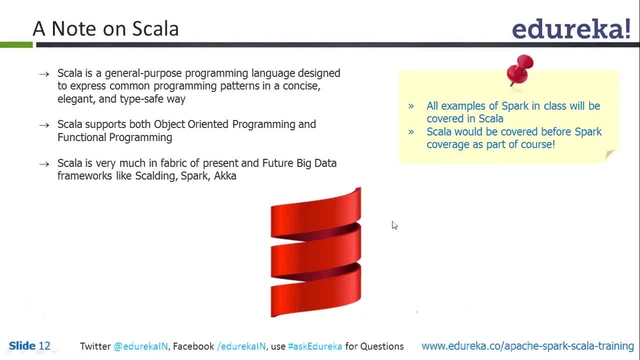 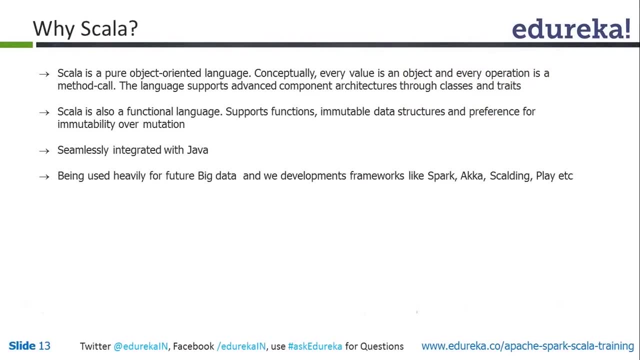 the other operations possible. okay, Now why Scala? again? I have to talk much about it already. that it's all about it is. it is a pure object oriented programming language as well as it supports a functional language, and, of course, the good thing is you can call Java code from Scala. 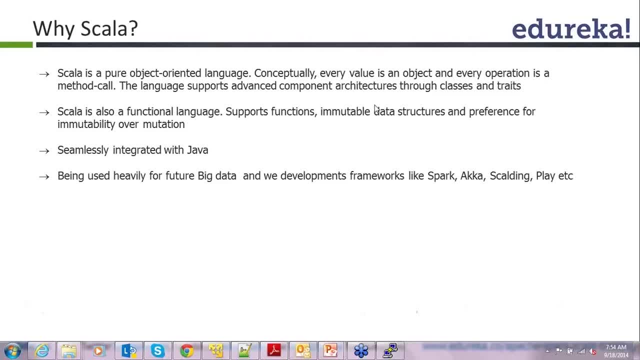 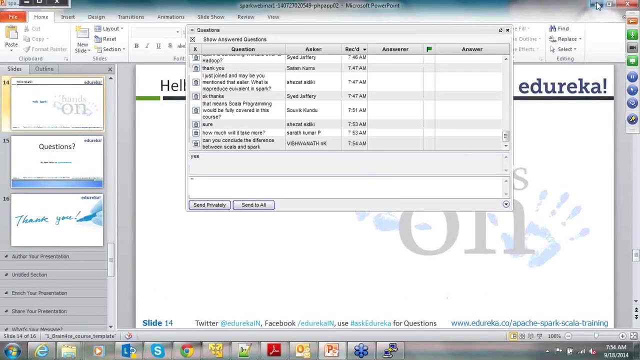 And vice versa as well. right, you can do all of that, yeah, and the- and of course it is going to be, you know, available in most of the future frameworks. that's fine, So no more time on this. So now I am actually coming to the point of showing you a small demo, okay. 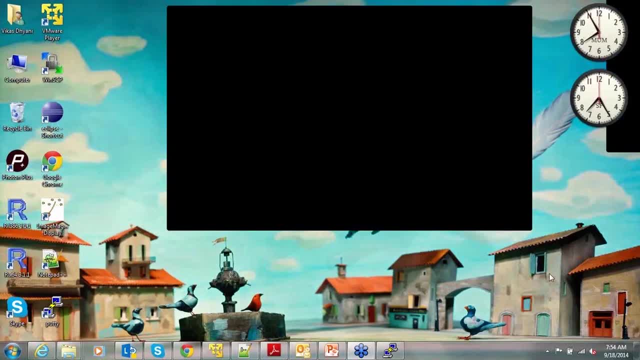 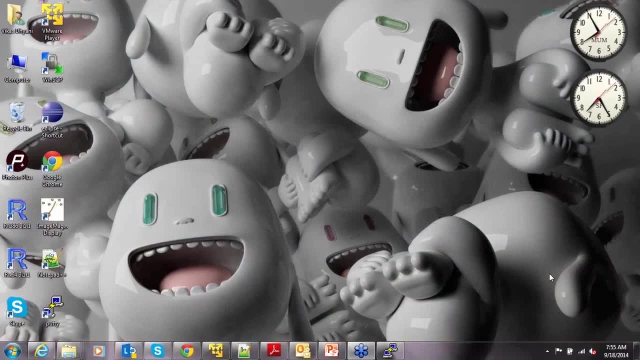 Where in I will be showing you a simple program which I will be first executing in a single Hadoop MapReduce, our typical Hadoop MapReduce, our every parameter will be the same means our input file will be the same. okay, And with Spark also, I am going to fetch the data from HDFS, though by default it fetches. 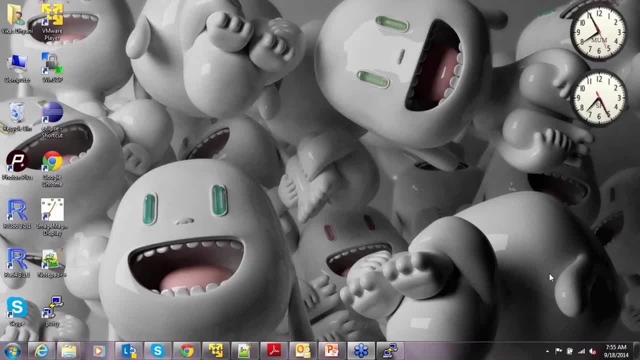 the data from local. but for just for this use case, I am going to fetch it from HDFS. all together, okay, And then you will first run it in MapReduce, That simple word, Come on, You know, right with word count. the good thing is, I don't need to tell many people what I. 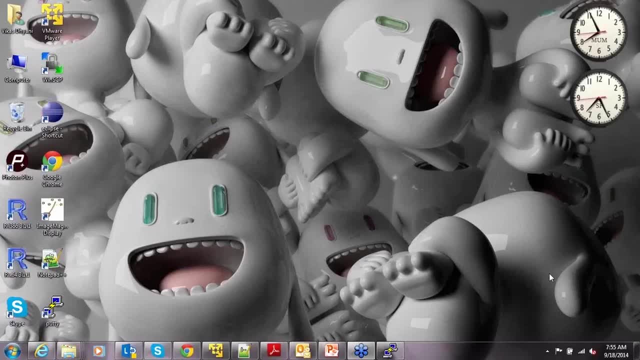 am trying to achieve, all right. So you will see that time and then very, very, very same file we are going to perform, or we are going to, you know, execute the Spark program on it, and then we will see the execution time Looks good, okay. 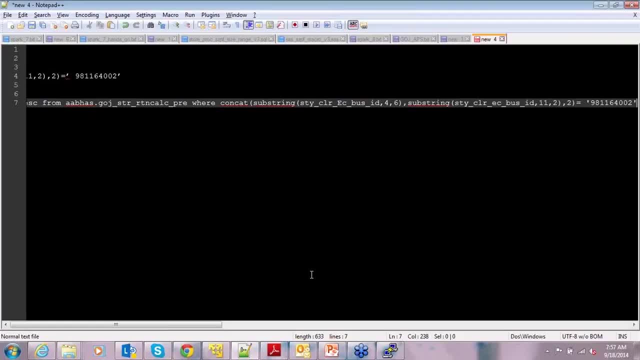 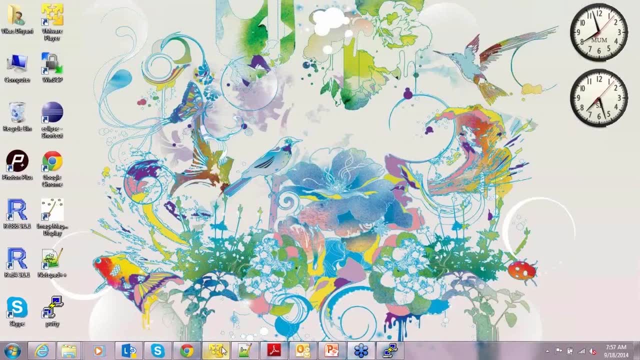 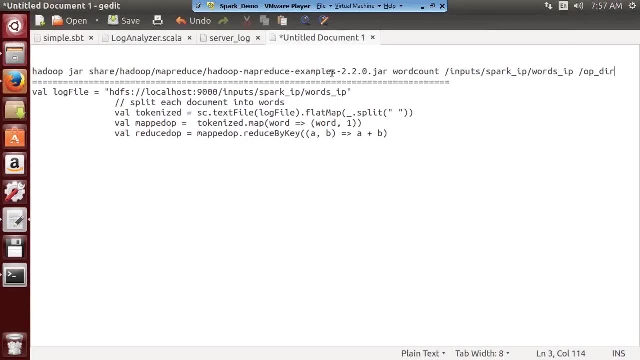 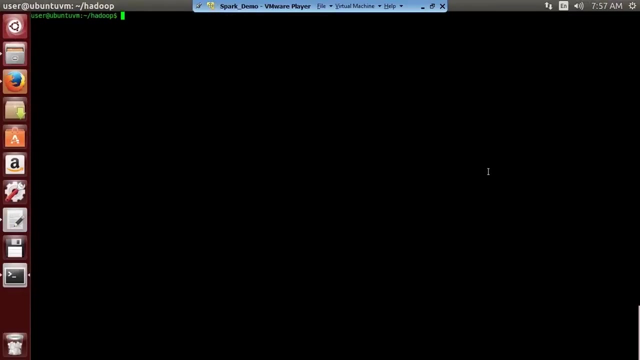 So let's, without wasting any time, let me just get started. sorry, some of my code files. So, guys, I am right now in Hadoop and just to save the time, first let me tell this is my HDFS thing. with Hadoop FS hyphen cat dual shift v, and let me just show you whatever. 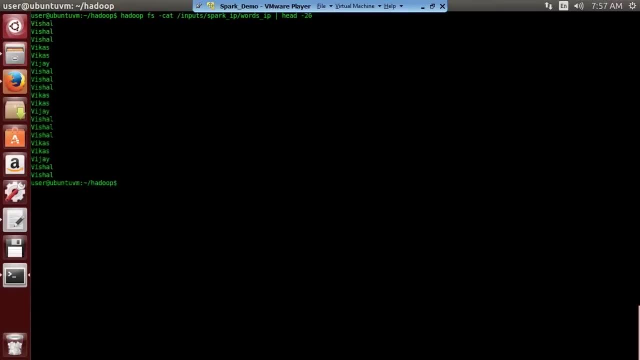 this is 20.. So this is showing you basically an input file which is having some words all together. So, just to tell you, I have kept only three names: Vishal, Vikas, Vijay- and they keep repeating over and over, again and again in this entire text file. 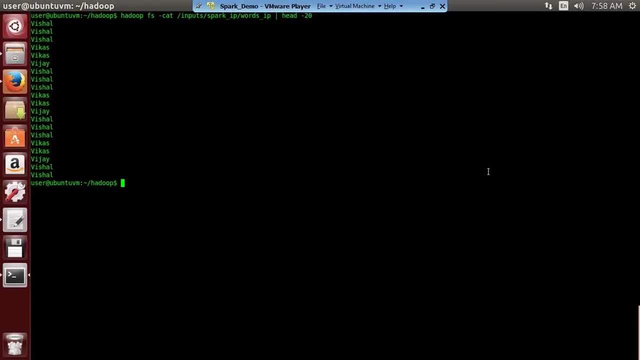 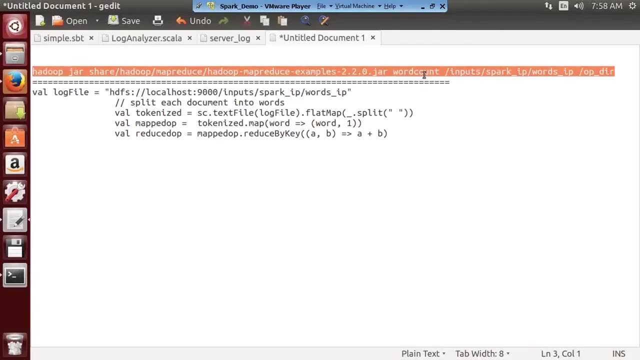 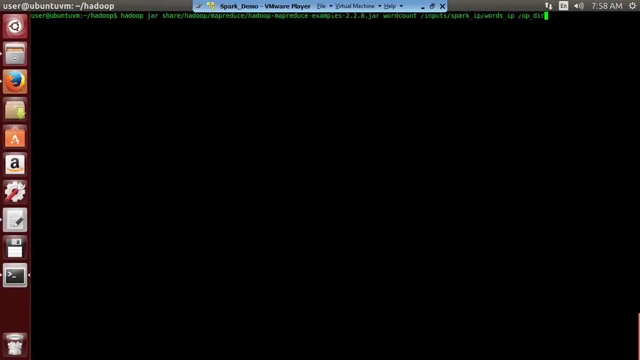 Okay, Now the word count is going to tell you which name has occurred how many times, right? So just to save the time and avoid any typo, I keep my commands ready, okay, So this is those people who are from you know Hadoop world. they know already, that's right. 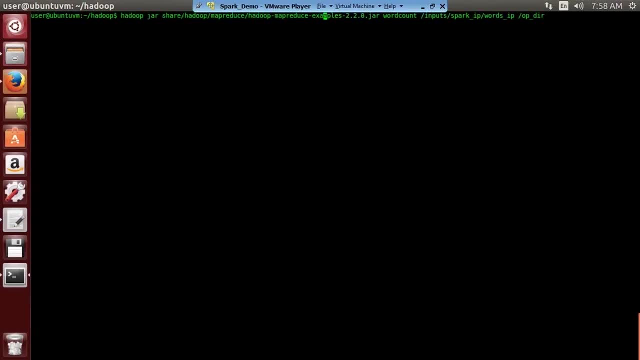 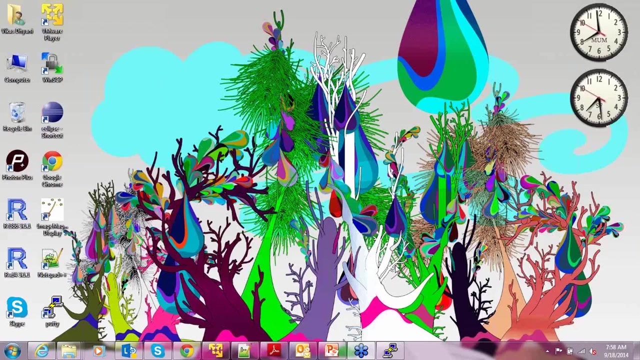 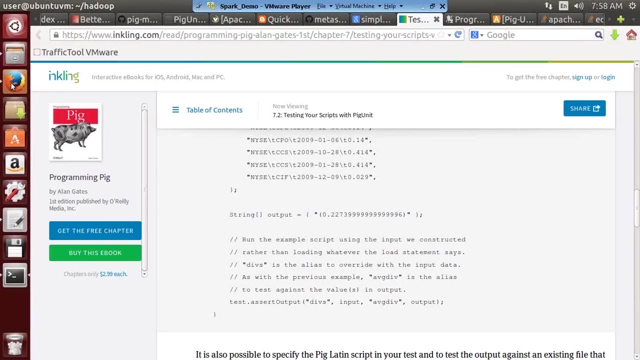 So Hadoop jar, I am running this inbuilt example. MapReduce example word count. this is my input. slash inputs. Spark input Word is underscore input OP. underscore DIR is the output directory where I am creating my output and let me run it. okay, sorry, now let me go. sorry, so many things. 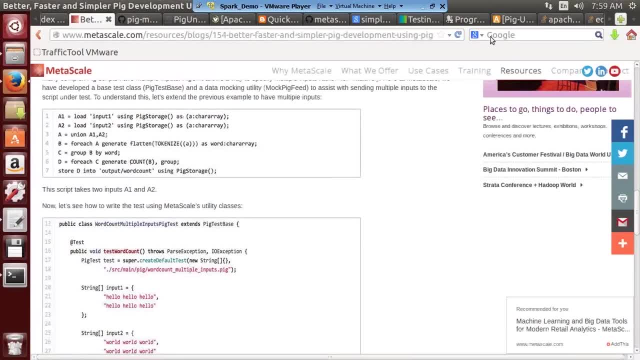 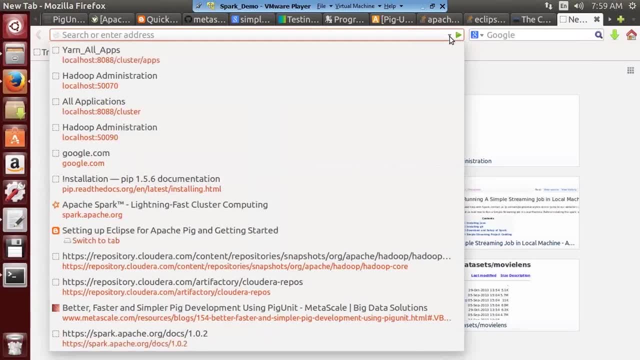 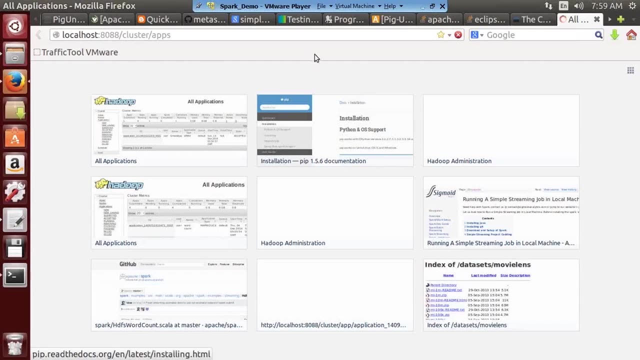 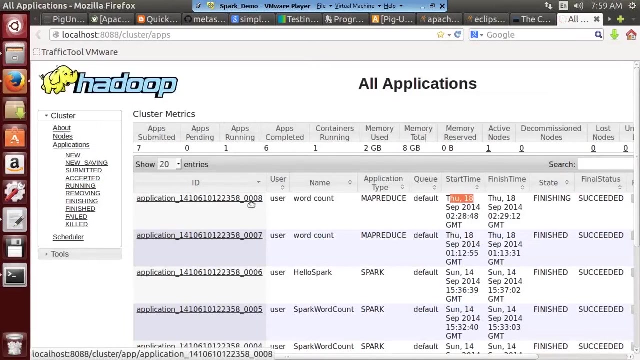 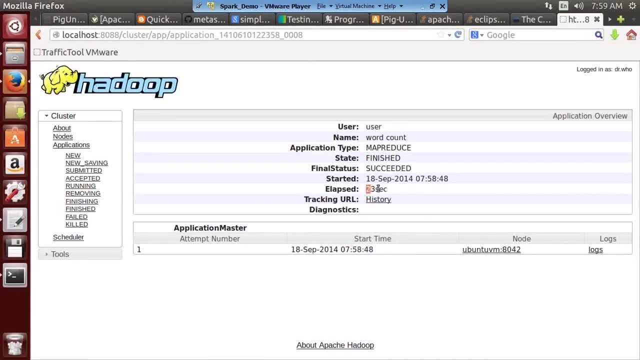 But it doesn't matter. Okay, Okay, Okay, Okay. have you seen this? what is the time which was taken? 23 seconds. you can see that it's quite fast, right? everybody has seen 23 seconds, right? let me show you the output as well, let? 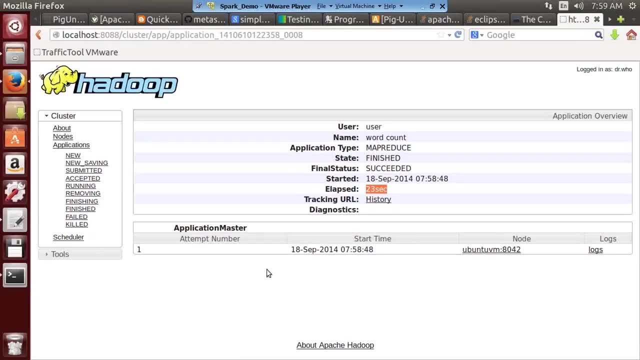 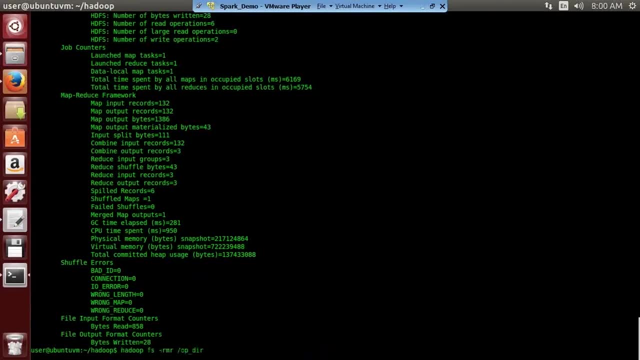 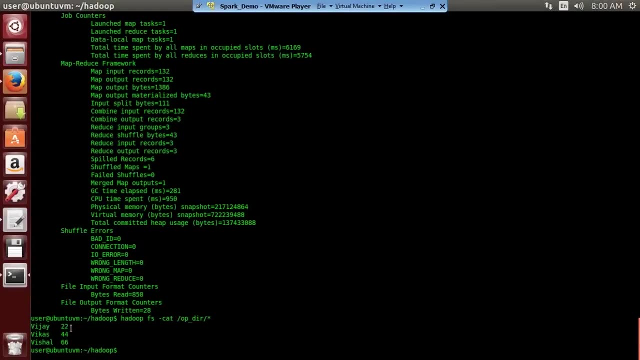 me show you the output as well. so the output of it would be Vijay 22, Vikas 44, Vishal 66. these are the frequencies of these words: Vishal appeared 66 times. Vikas appeared 44 times. Vijay appeared 22 times. 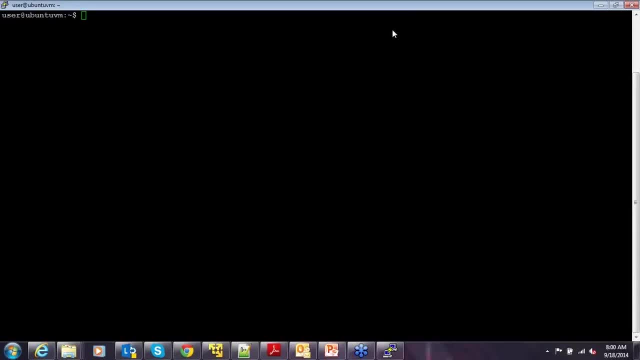 right guys, are we good with this park exam? sorry, with this. with the Hadoop example, wherein it's a simple word count, we have seen that it takes 23 seconds and we got the output as well. right now, let me run the very same example in spark, so in. 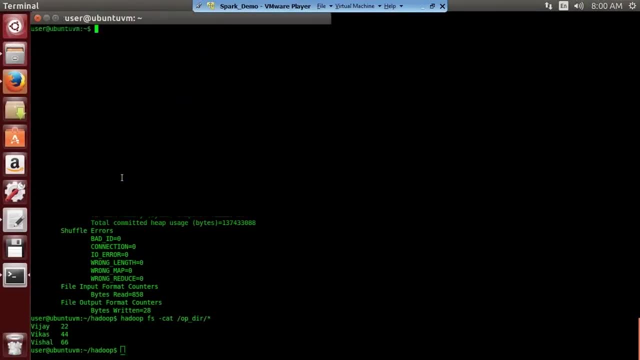 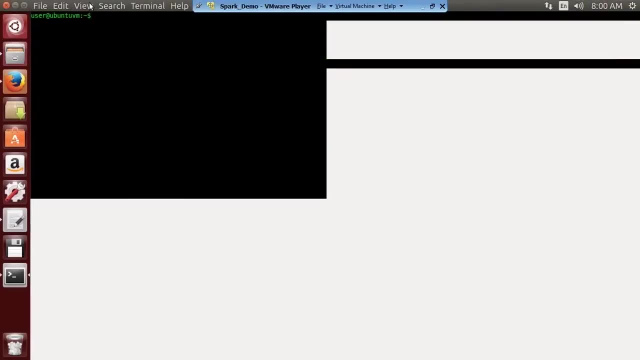 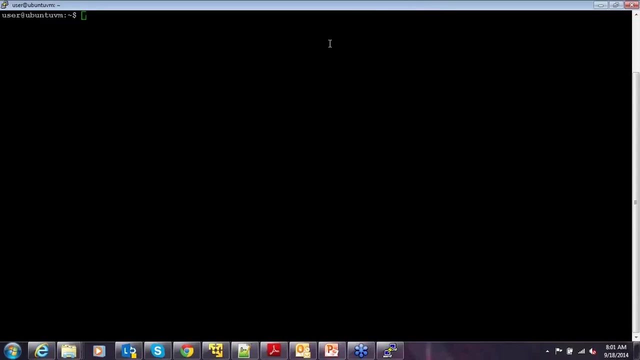 order to do that, I will open under terminal- okay, come on- rather than doing it here. so this is putty through which I am capturing my machine, just for a better view. nothing else. spark- this is my typical that spark directory. I will go and fire up the spark shell. 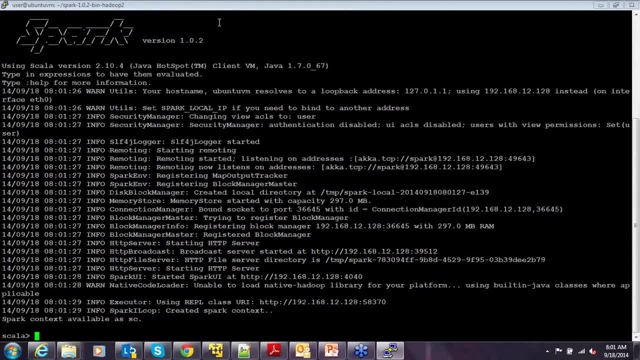 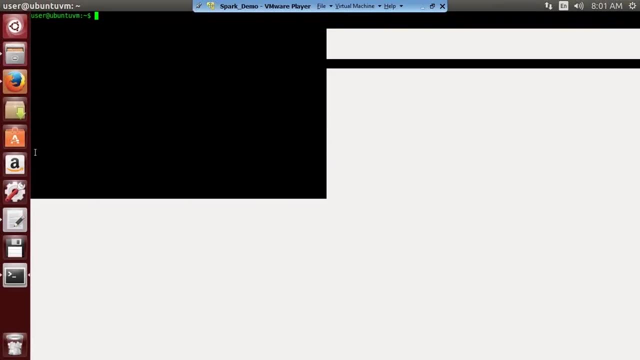 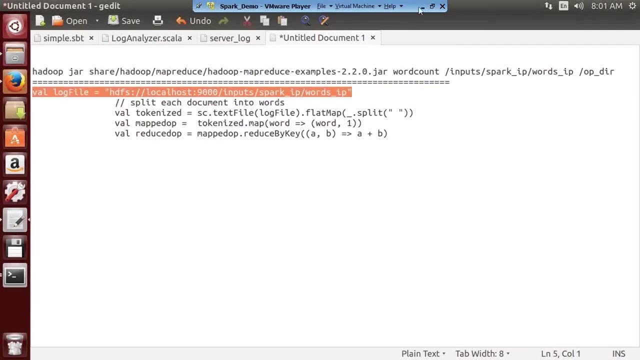 okay, so I fired it up. now it has basically so by default, it gives you that Scala rappel altogether. now let me just run my instructions to it. it's kind of interactive. so first thing is, I'm not explaining the meaning of each and every. you know each. 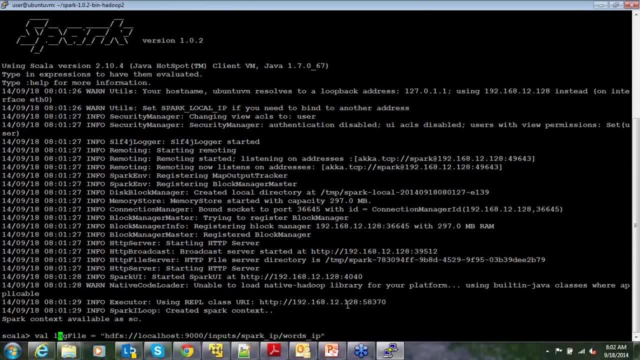 and every of my statement altogether is: you can just see that well log file. you can see this. I am fetching the data from his Davis and you can see that slash inputs, spark input words: input, it's the say. it's the same input which I have taken for my map: reduce job. 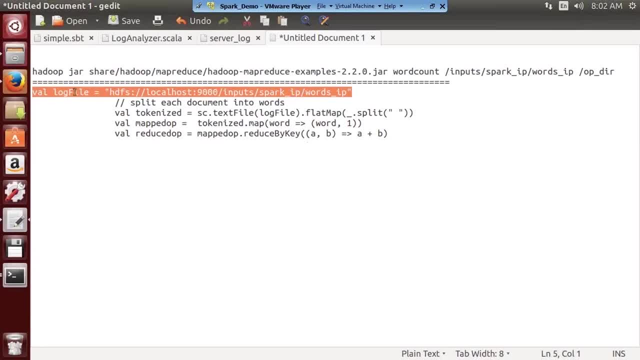 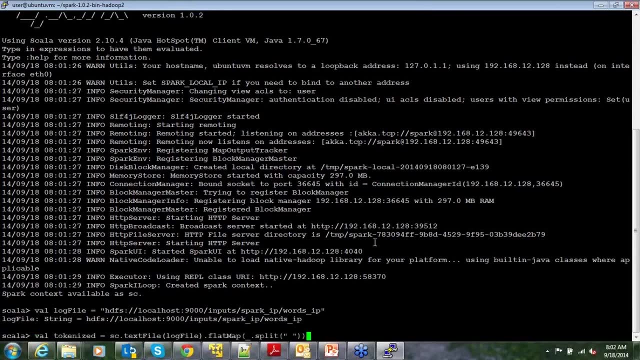 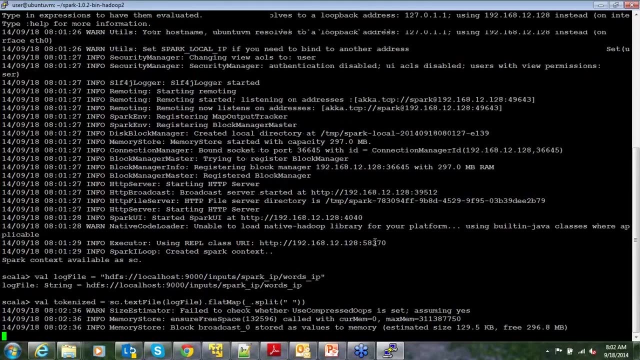 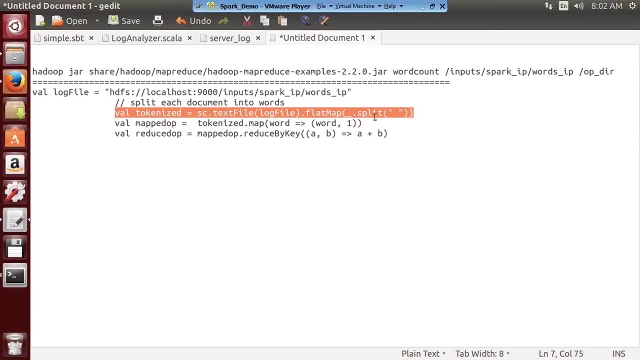 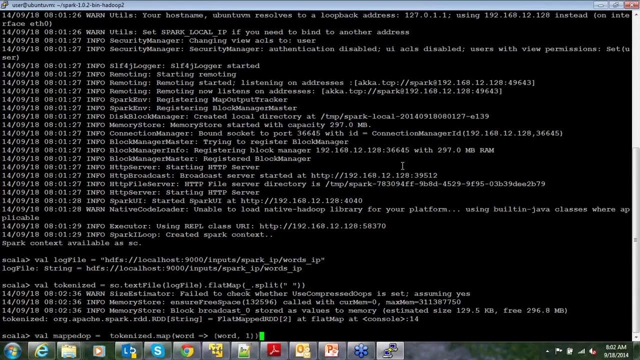 then now. so I'm not going to explain much about this right now. I'm just just to tell in my produce terminology, I'm doing the tokenized operation. okay, so these are some tokenized operations which are happening. then this is the map stage. I could have achieved all of this in a single line, that's on the beauty of Scala. 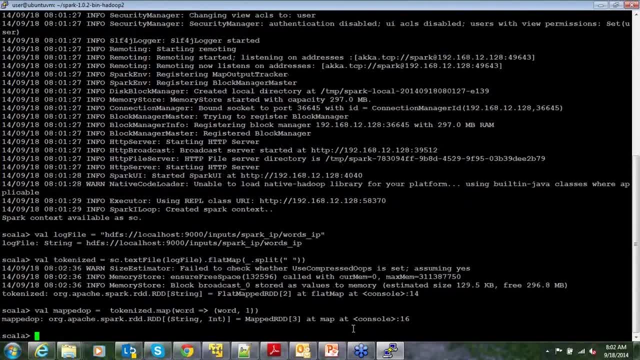 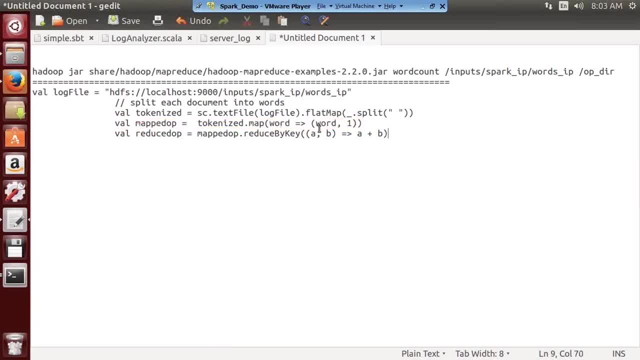 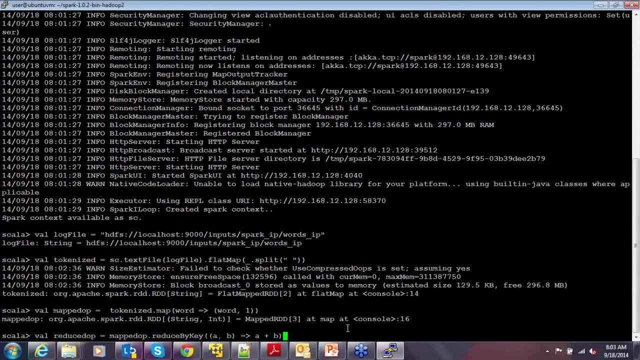 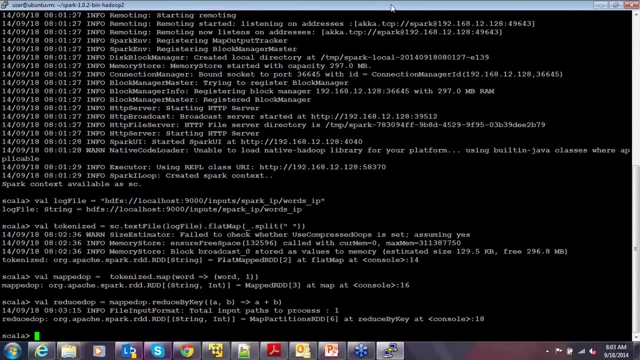 and right now you can see that some of the things are happening, but no actual calculation. this is like logical way. Scala- is this basically a spark- is just ready to perform the calculation, but it has not really performed anything as of now. okay, this is the reducer side output, so when you run it, there is no output here at. 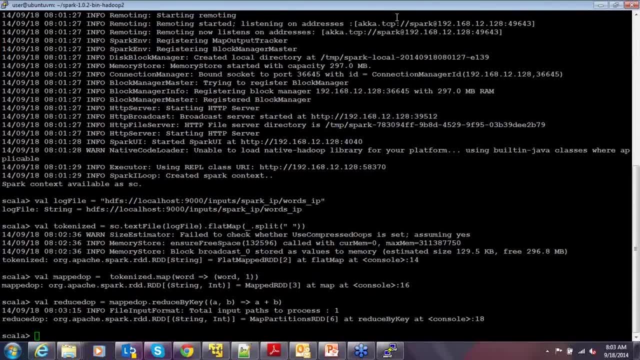 such as of now, because all of this, okay, all of this is something which is kind of calculated, not really. I mean sorry, a kind of you know, a DAG is prepared but no actual calculation is forced. now, when I try to say reduced op dot collect, now the calculation would happen. 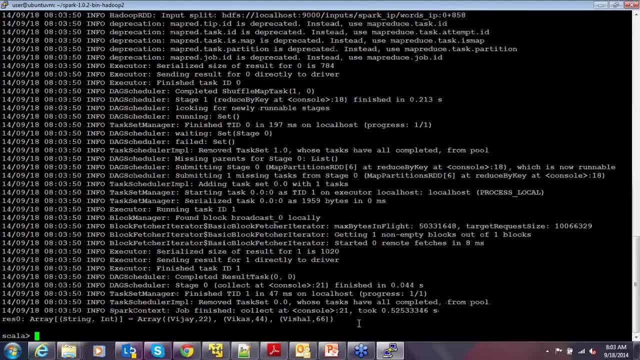 so let me run it over. see the output: Vishal 66. Vikas 44. Vijay 22. can you see more than this? can you see the time? you saw 26 seconds and then you are seeing 0 point 0.044 seconds. it is right in front of you saw that everybody: 0.044 seconds altogether. 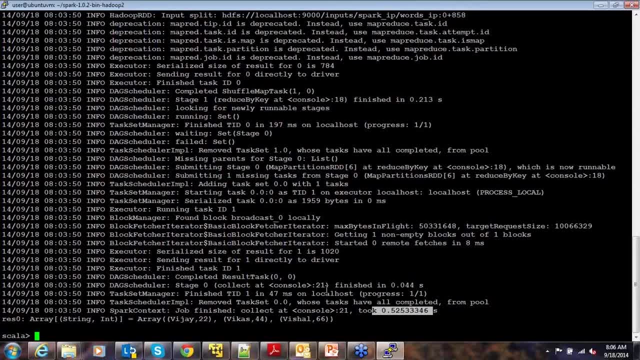 so now it is up to you to see that. what exactly is the difference which you saw? it is the same word count. I didn't do anything right. it is the same word count. optimized one, not written by me, right. pre-shipped example takes 26 seconds. 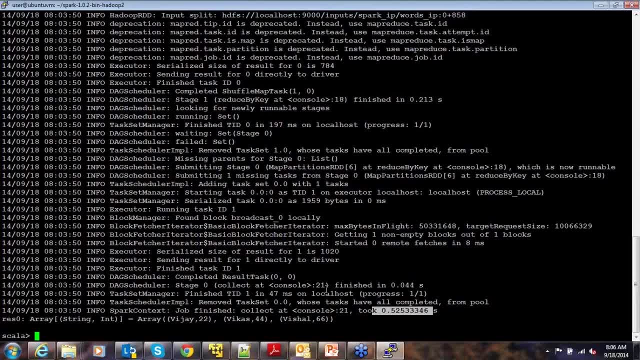 On the same data set and the same one in spark takes less than a second right guys. so with this my coverage for the session ends, and I just hope that you found it useful. thanks a lot for attending it. logging off now, do provide your feedback, guys. 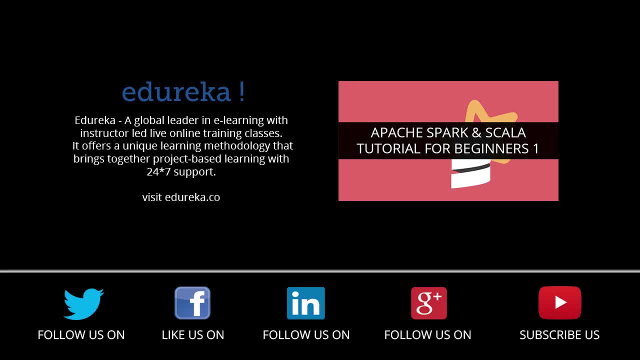